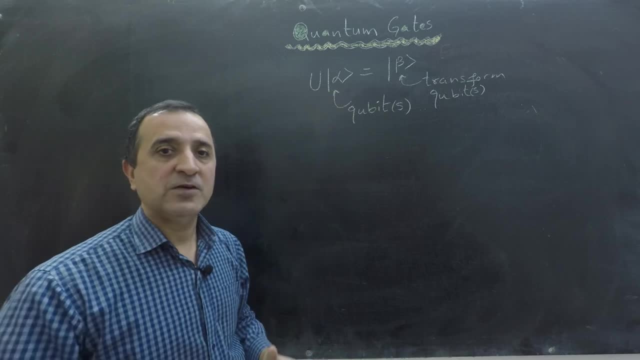 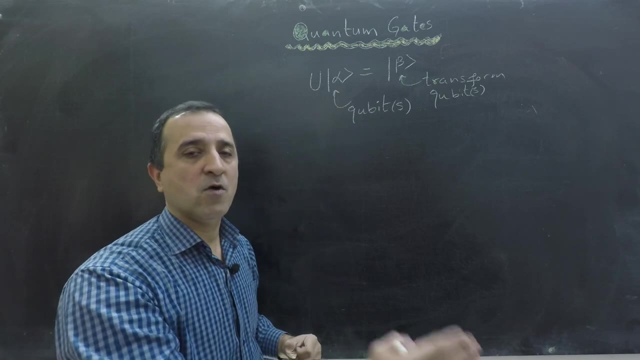 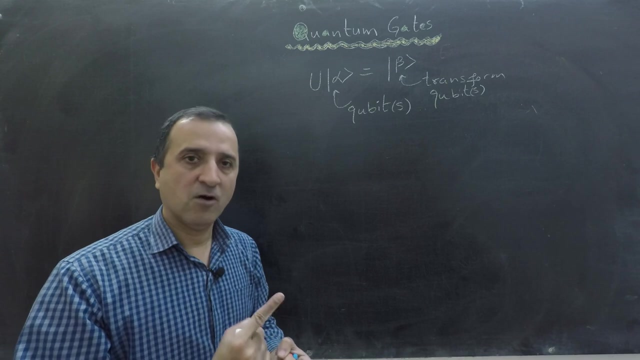 This operation u is equal to the sum of probabilities for qubits. This operation? u must be special, which preserves the sum of probabilities. That means this operation? u must preserve the norm of a vector, And that's why we know that there is only a single type of operation, a single type of matrix. 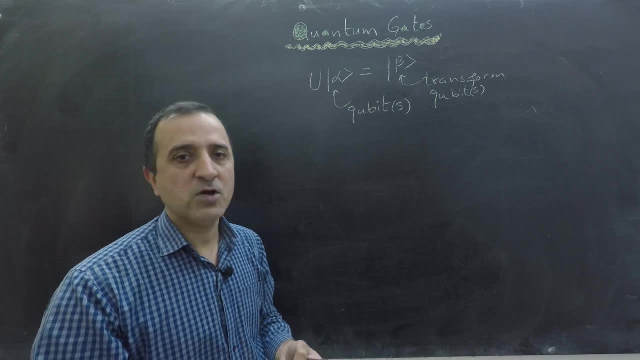 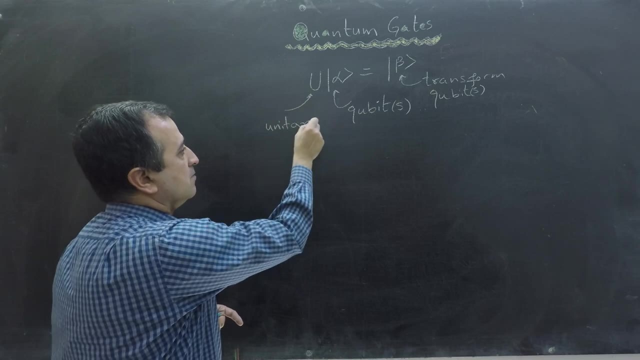 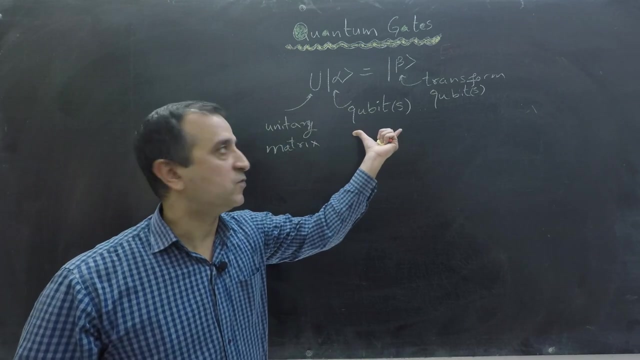 that can preserve the norm of a vector which is called a unitary matrix. So this must be a unitary matrix, Because otherwise we will say here the sum of probabilities equals to one And the transform qubit has sum of probabilities equals to ten, which will be wrong. 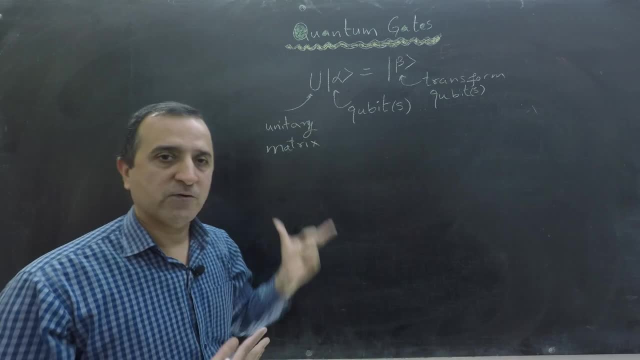 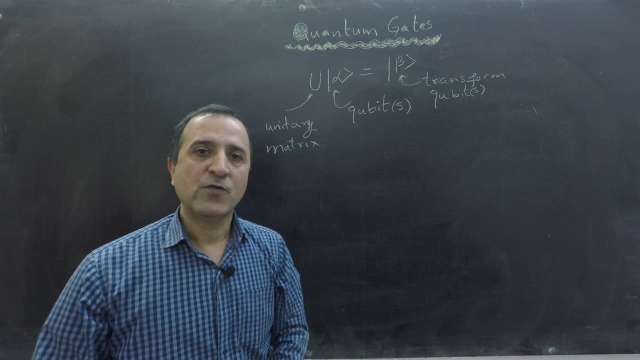 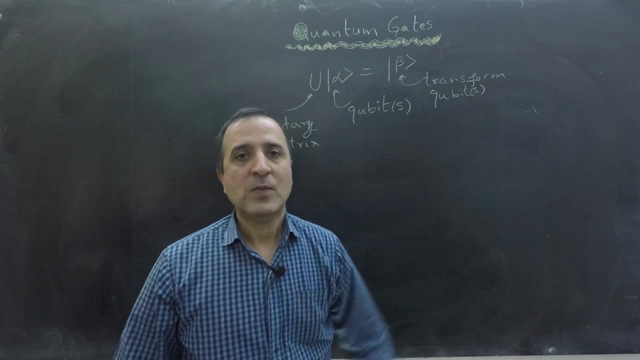 So only the unitary matrix are the types of matrices that always preserve norm of a vector. I have made a separate video proving some of the simple properties of unitary matrix. The link of that video will be somewhere here, So please watch that video also to become a better scientist. 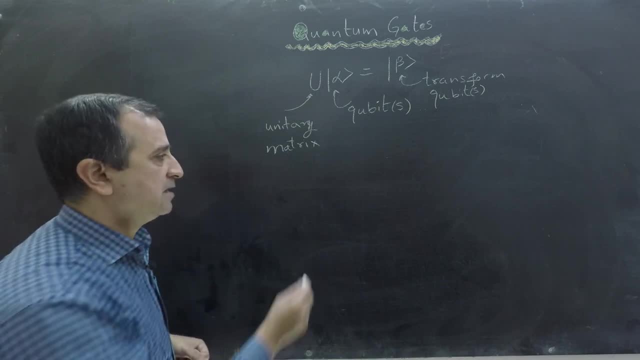 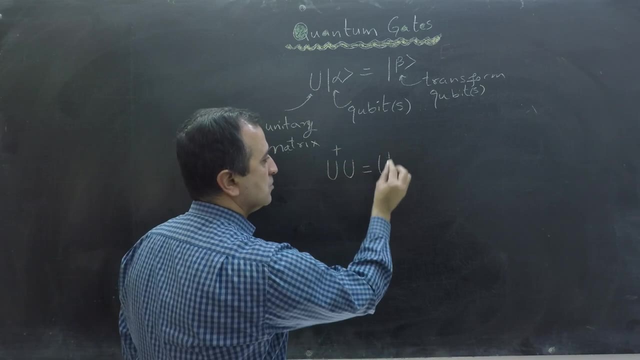 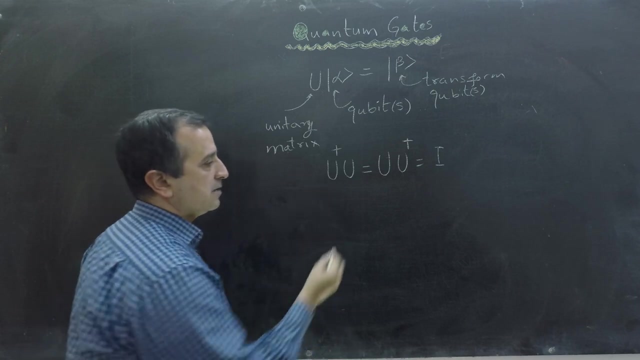 Now, what is a unitary matrix? A unitary matrix is where u conjugate transpose times u is equal to u. times u conjugate transpose is equal to identity. So you can say that in this case my conjugate transpose is basically the inverse. 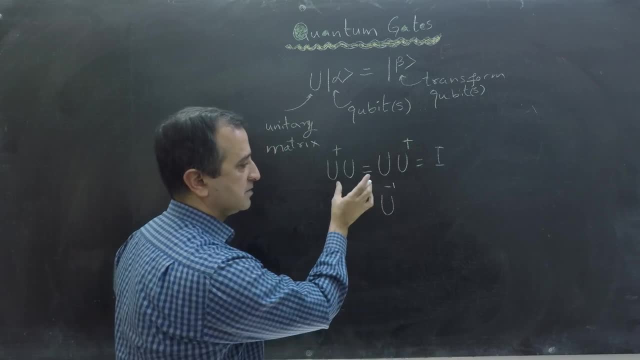 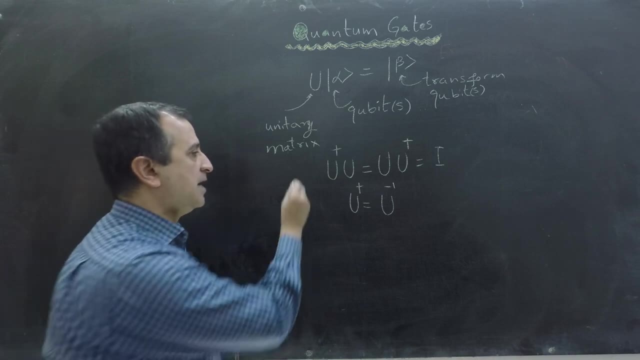 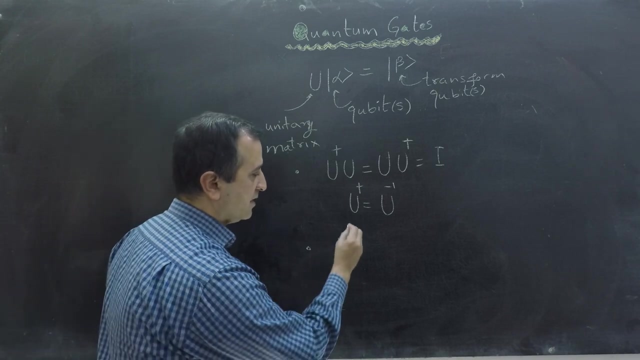 So if I take conjugate transpose of a matrix u, I will get its inverse. Now there is another kind of matrix called Hermitian matrix. For Hermitian matrix, if I take conjugate transpose, then my result is equal to the same matrix. 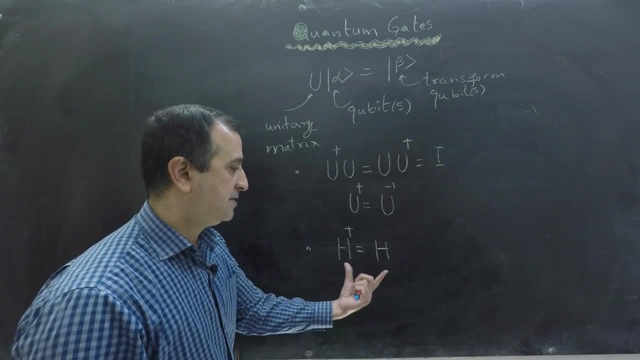 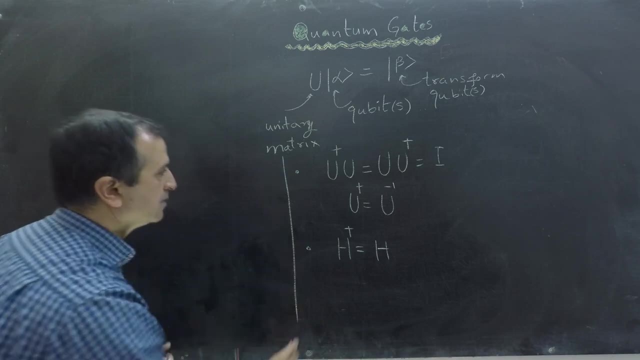 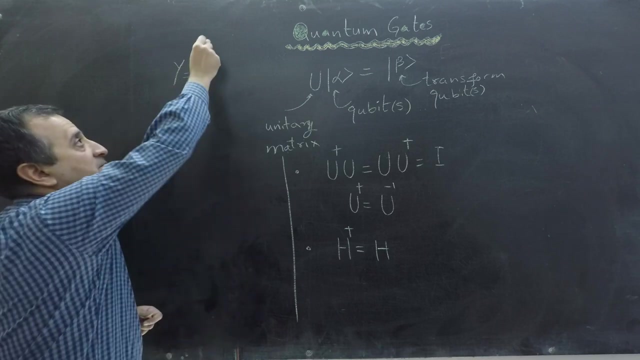 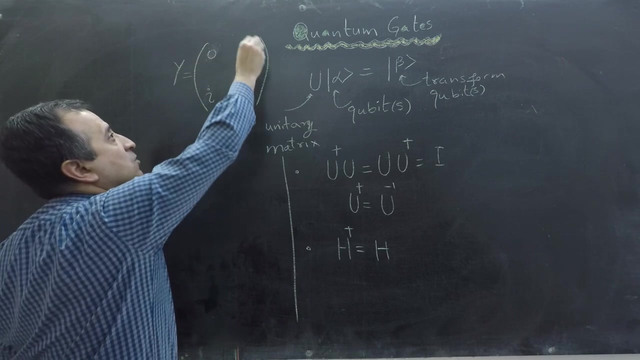 So conjugate transpose doesn't change the result and my result is equal to the same matrix. Let's do an example to make it clear. In this example, my matrix is called y And the matrix is 0 iota minus iota 0.. 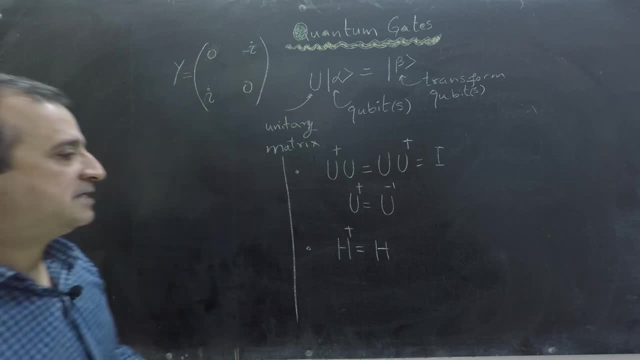 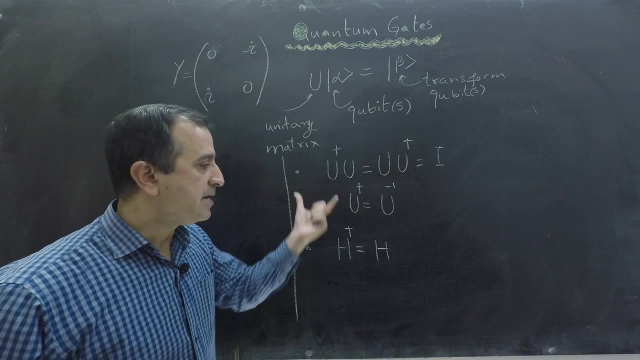 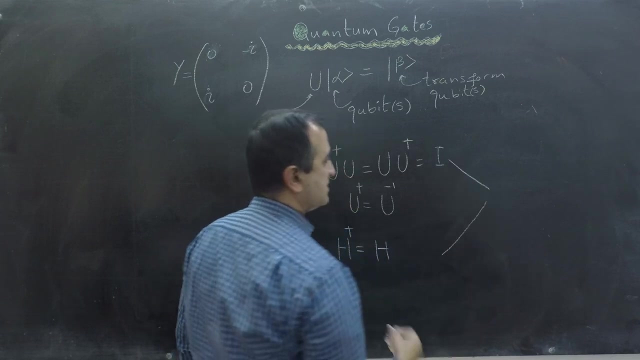 Now I have to verify if this matrix is unitary, Hermitian or both. By the way, if a matrix is unitary as well as Hermitian, then it has a special property that in this case, its inverse is equal to itself. 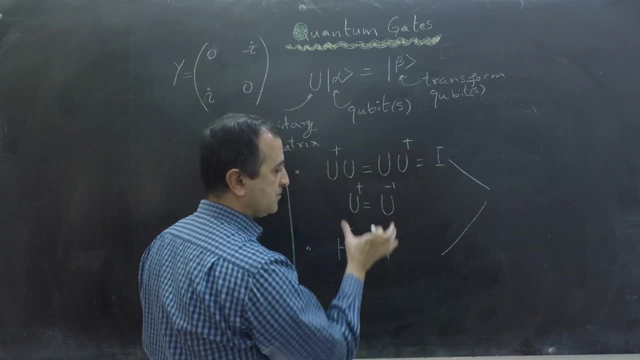 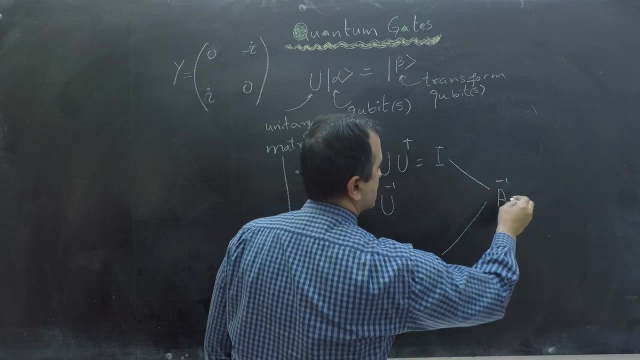 Because of these two properties, when combined together, we can say for this matrix: if this matrix is a, then its inverse is equal to itself. We don't have to take conjugate transpose, We can just multiply that matrix with itself and we will get identity. 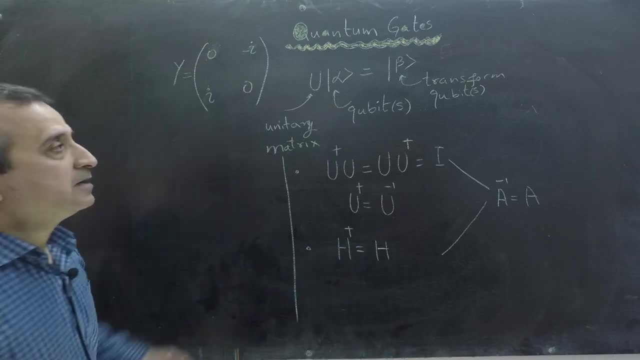 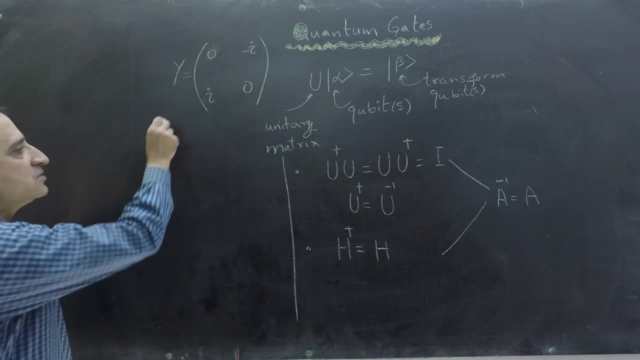 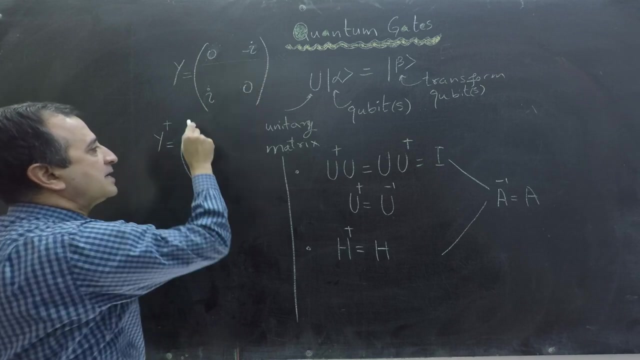 And this matrix here is unitary. Unitary as well as Hermitian, So let's try. So if I take conjugate transpose, then my answer is that first I take this row and write it as a column, So 0 minus iota. 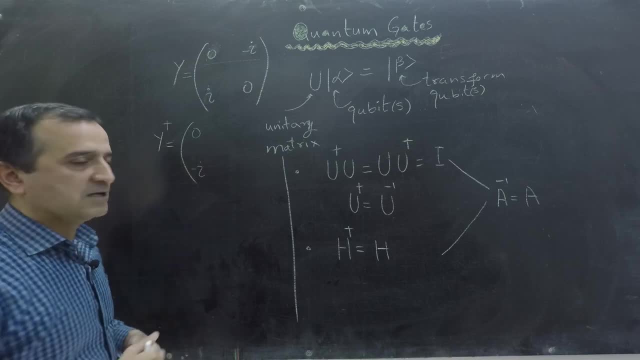 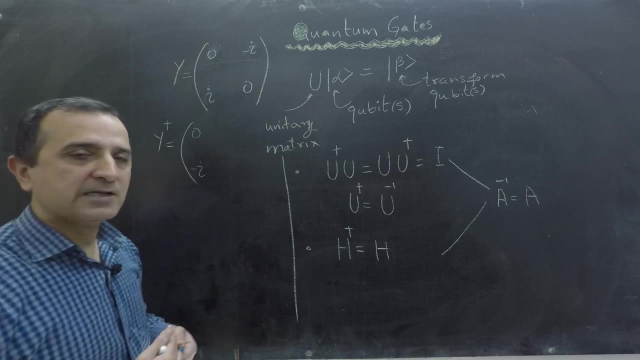 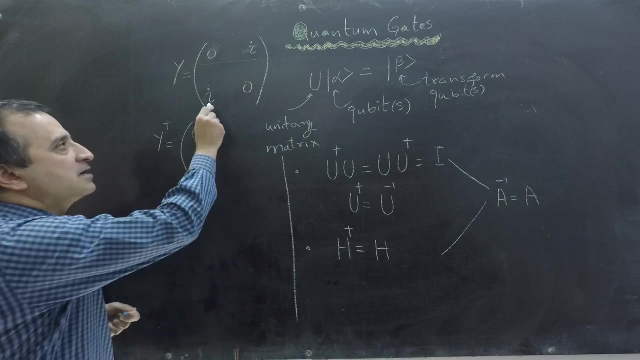 But I also have to change the sign of all the terms having iota, because I have to take, transpose and also conjugate, And conjugate implies that the terms having iota change their sign, So this iota will become plus iota. Now take this row and write it as a column. 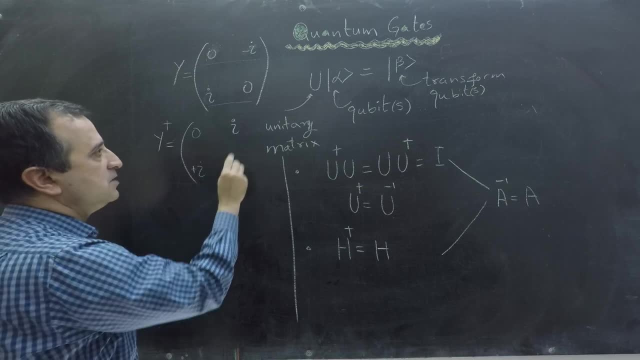 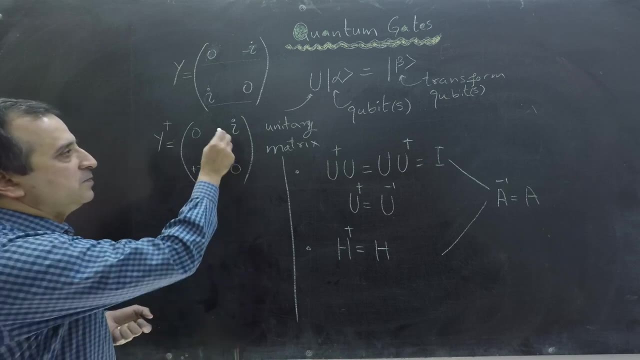 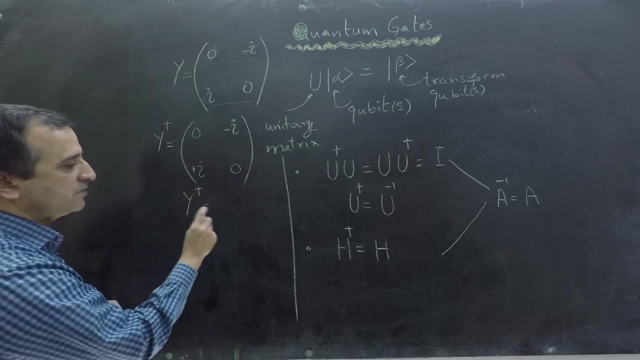 I will get iota and 0. Once again I have to change the sign of all the terms having iota, So this will become minus iota. And now you can see that conjugate transpose is equal to y, So y is the Hermitian matrix. 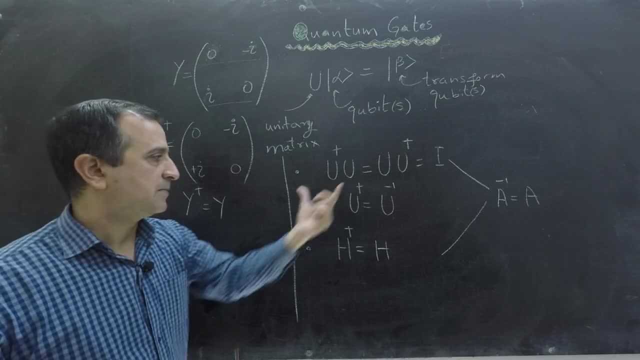 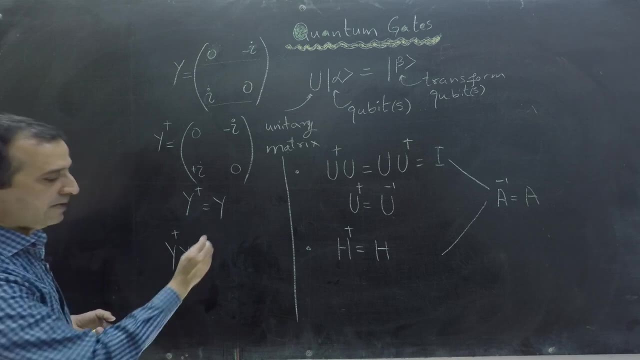 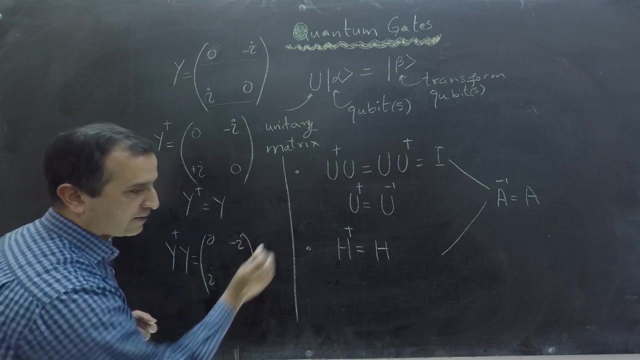 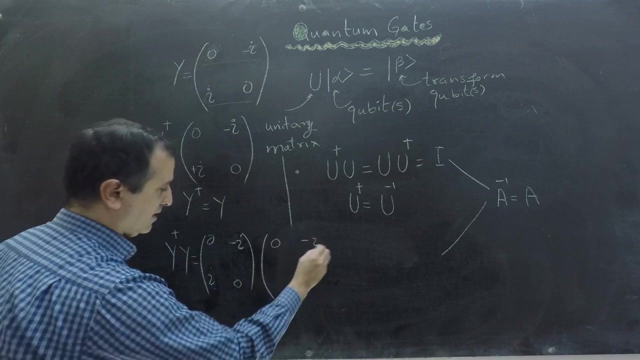 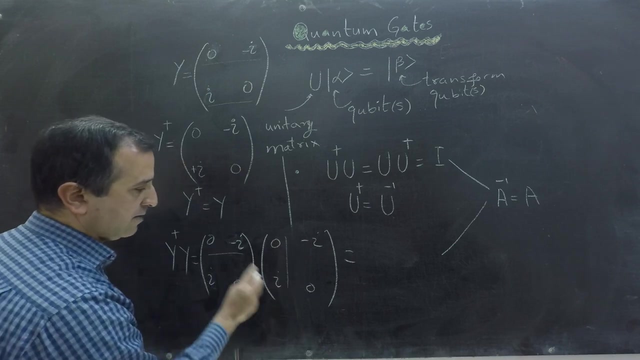 Now we have to see if this is our unitary matrix. To that end, we multiply y conjugate transpose with 5.. So we multiply 0 minus iota iota 0 with 0 minus iota iota 0.. And this will be 0 times 0. 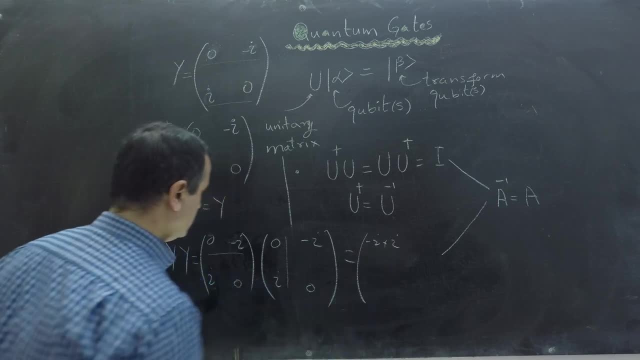 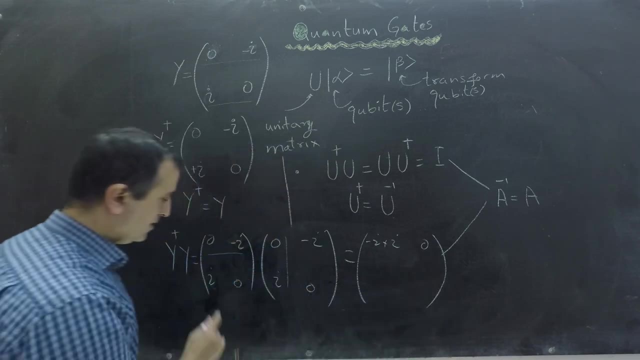 And this will be minus iota times iota here, And then this will be 0 times this, And then this will be 0.. So I will have 0 here, And then here I will have 0 plus 0.. So I will have 0 here. 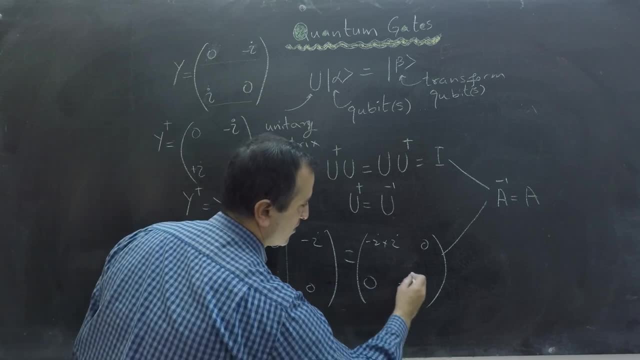 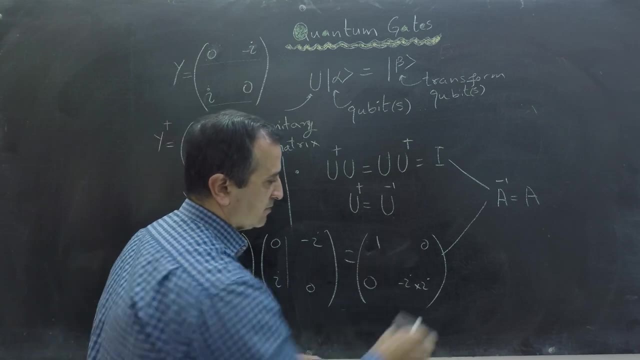 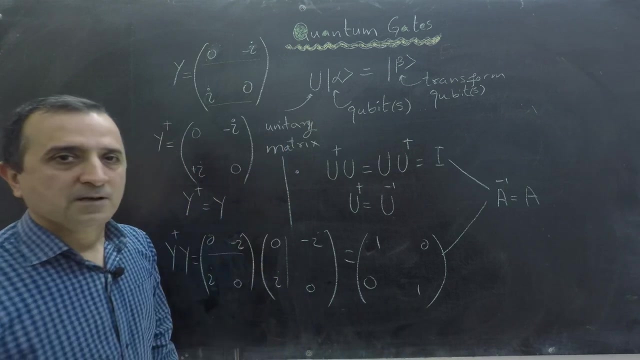 In the last case, I will have once again, minus iota times iota, And this simplifies to 1.. And this simplifies to 1.. So yes, this matrix is both Hermitian and unitary. Now, after explaining these simple concepts, 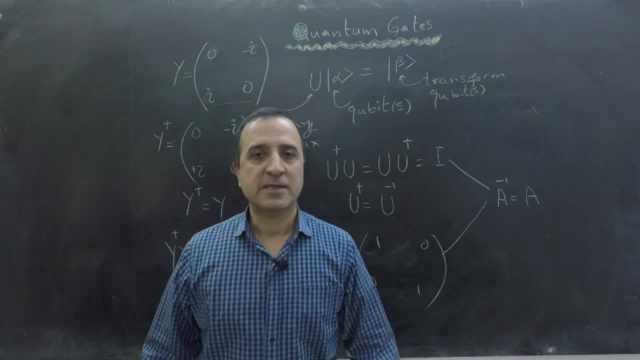 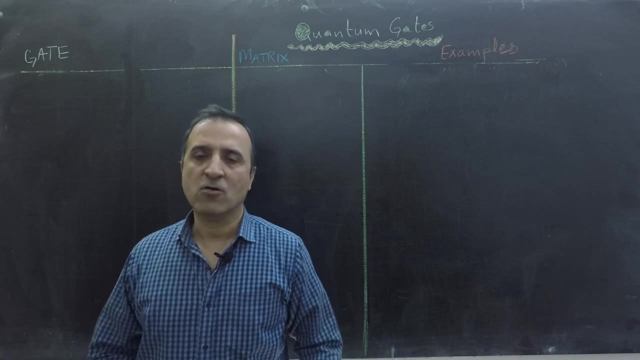 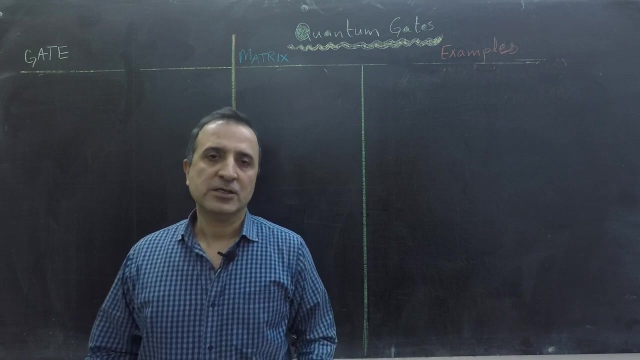 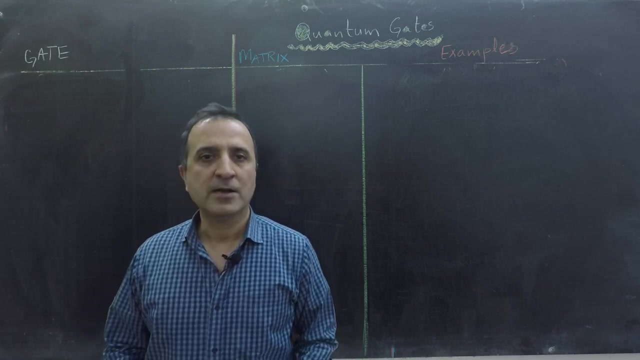 we can now list the quantum gates. Now we can list some quantum gates. Obviously, there are infinite many quantum gates because there are infinite many unitary matrices And each unitary matrix can be considered as a quantum gate. However, in this video I will write most widely used quantum gates. 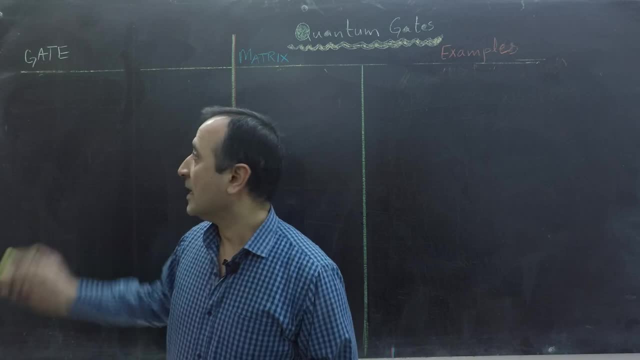 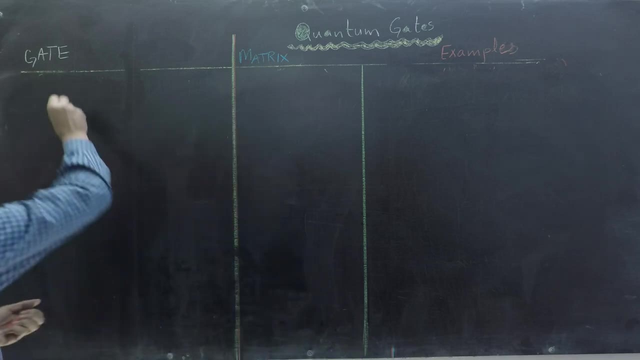 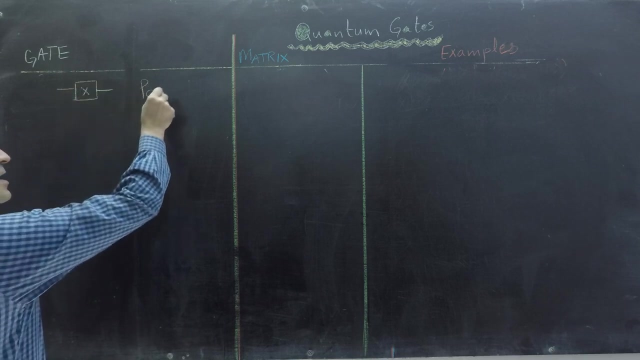 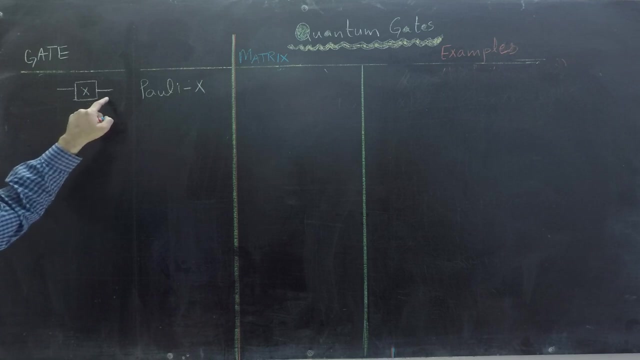 Let's start with the x-gate, which is also known as poly x-gate or not gate. Poly x-gate, Poly x-gate takes a single qubit s input and produces a single bit s output. Like all quantum gates, it is reversible. 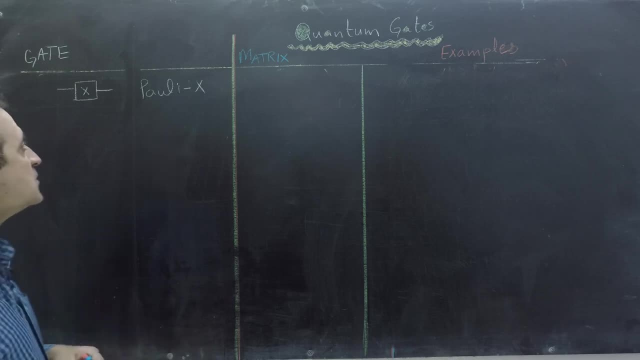 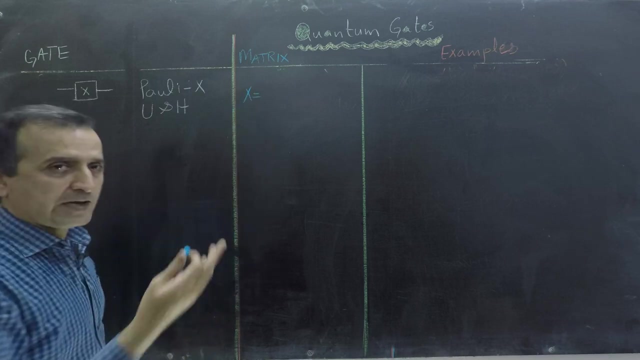 and it is reverse of itself. It is because this gate is both unitary and Hermitian. All the gates which are both unitary and Hermitian are inverse of themselves. Now let's write the matrix of this gate, So matrix of our x-gate, or poly x-gate or not gate. 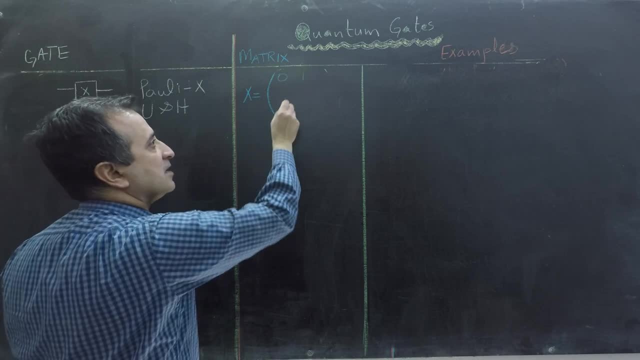 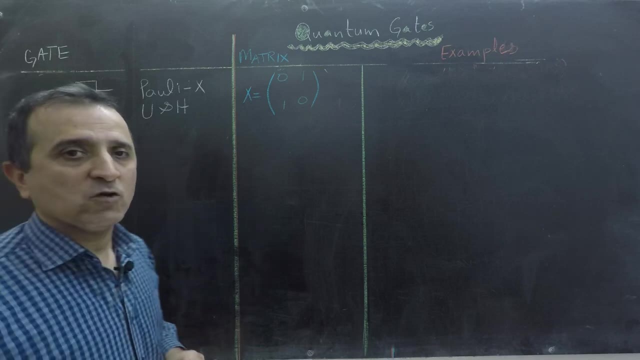 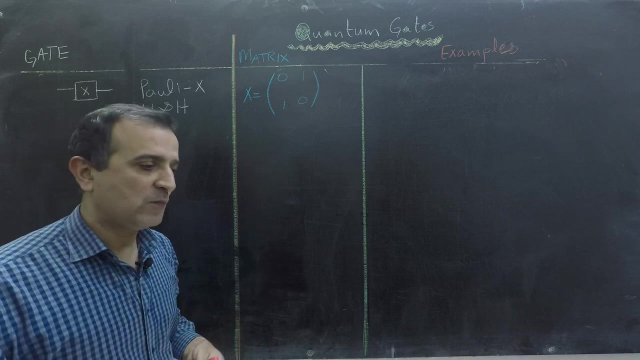 is equal to 0, 1, 1, 0.. Now please note that for a single qubit we need 2 raised to power 1.. That means 2 by 2-dimensional matrix, because single qubit needs a 2-dimensional vector. 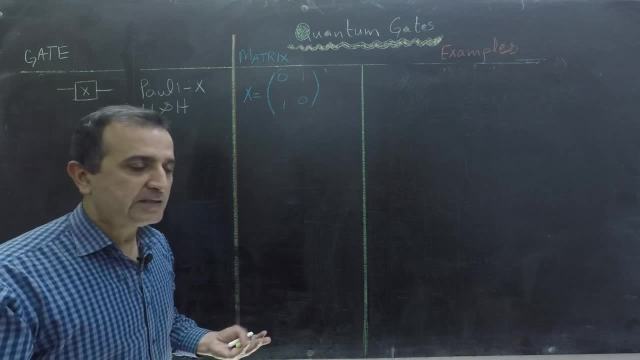 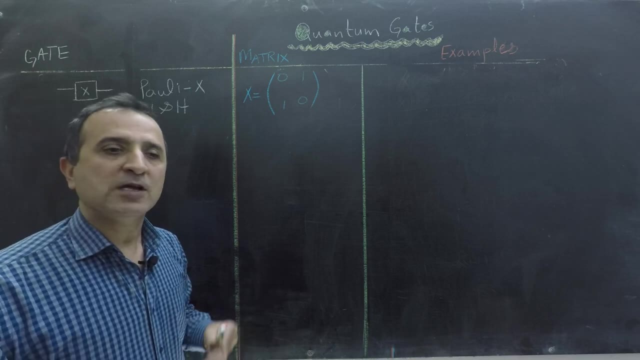 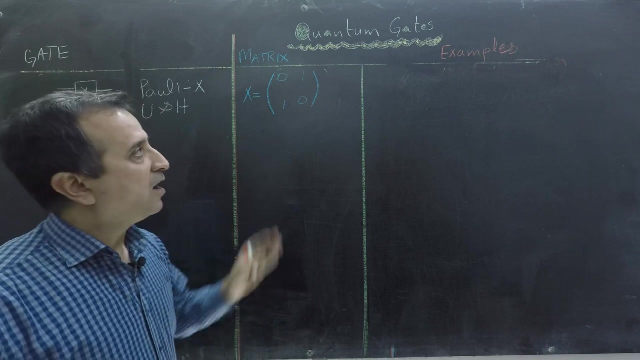 for its representation And for 2 qubits we need 4 by 4-dimensional matrix, And to manipulate n qubits we need 2 raised to power, n by 2 raised to power- n-dimensional matrix. Now let's see how this matrix operates. 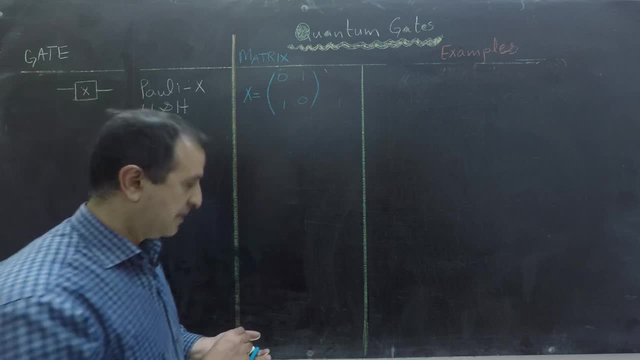 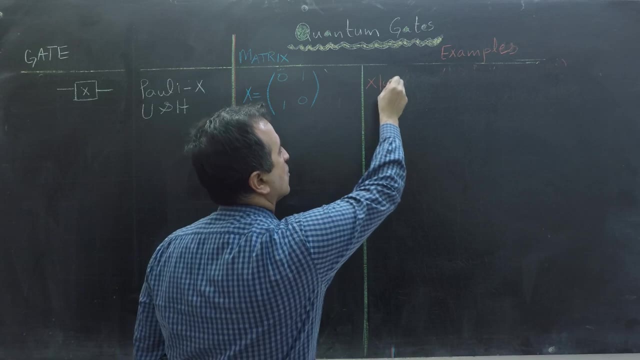 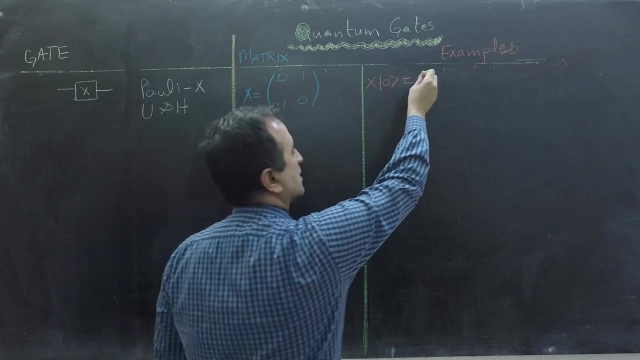 on different kinds of qubits. Let's say I take my quantum gate x and apply it on a pure state of ket 0. Then it alter the state of the qubit from 0 to ket 1, because it is a node gate. 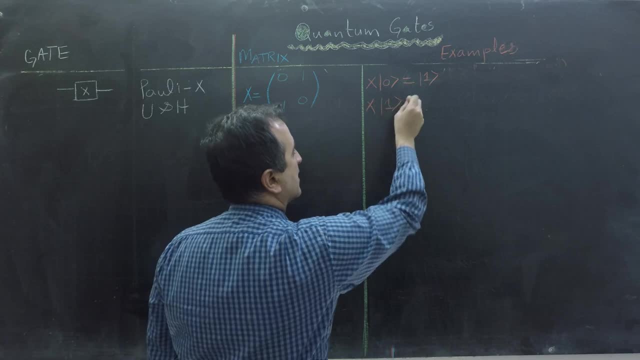 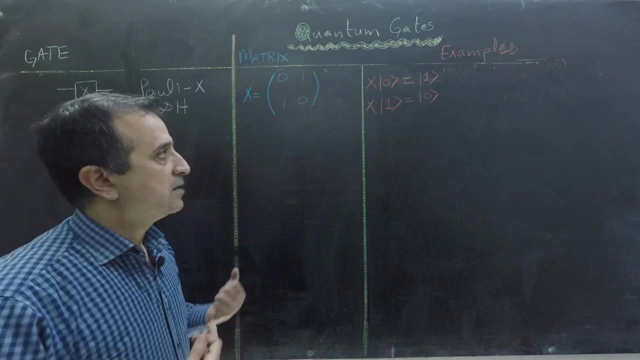 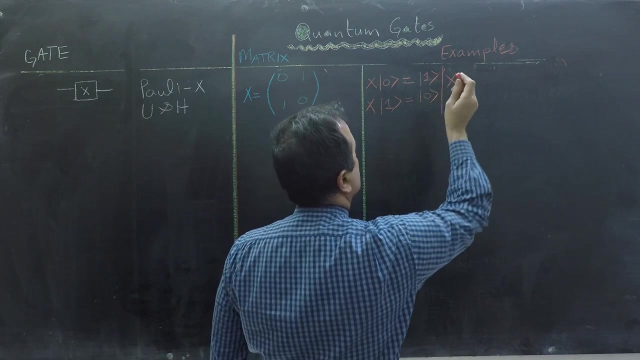 Similarly, if I apply it on ket 1, my answer is ket 0.. I think a more interesting case is that I apply x-gate on a superposition. Let's say I apply x-gate on a superposition of alpha, ket 0. 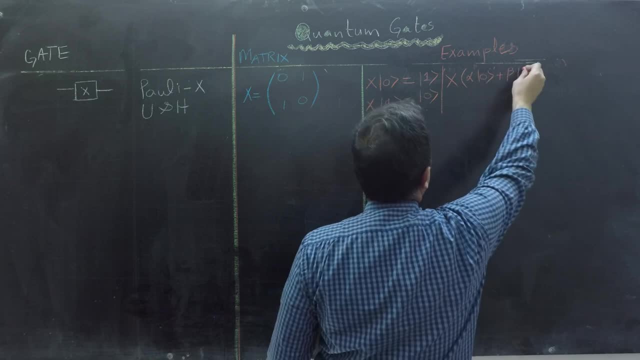 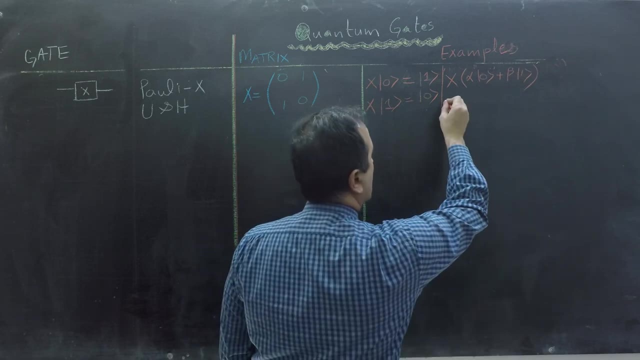 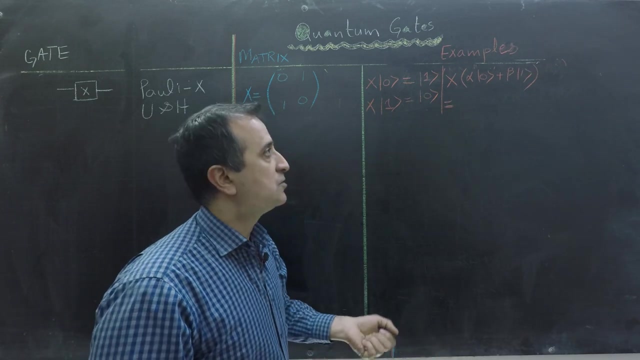 plus beta, ket 1, where alpha and beta are complex numbers and they normalize this vector. So how to find our answer Now? note that all the quantum gates are linear, So we can simply take this x inside the summation and rewrite it as: 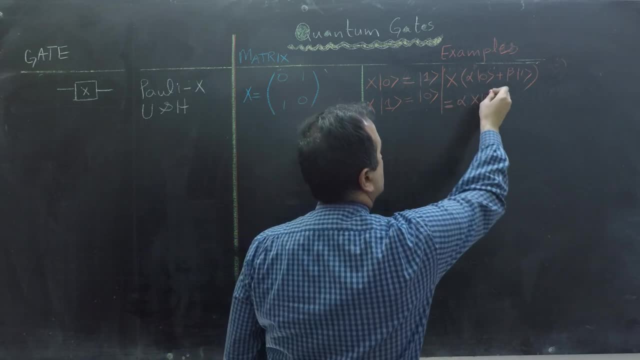 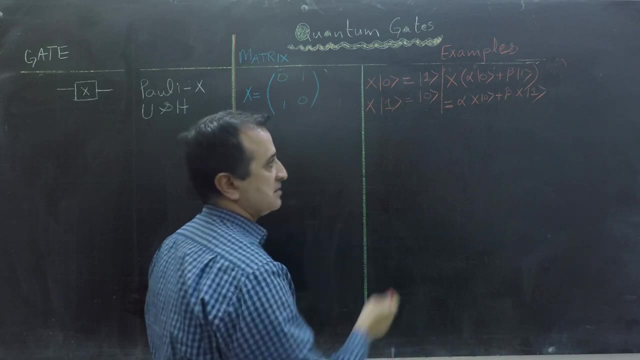 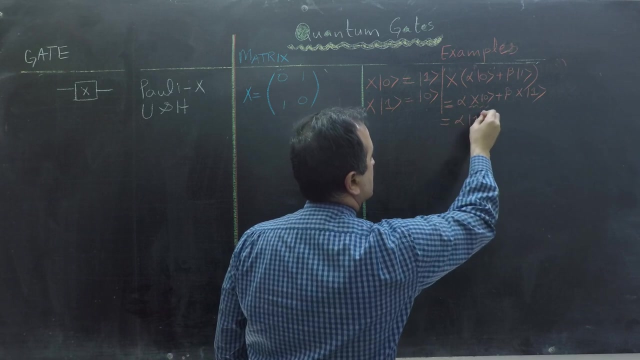 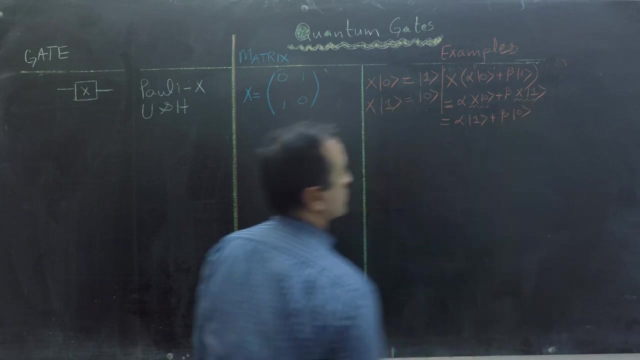 alpha x times ket 0 plus beta, x times ket 1.. And now we can simplify it easily to alpha, and this will become ket 1 plus beta, and this will become ket 0. So now we know how to apply our x-gate on pure states. 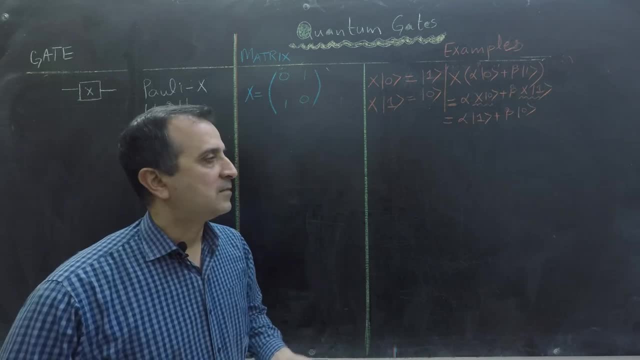 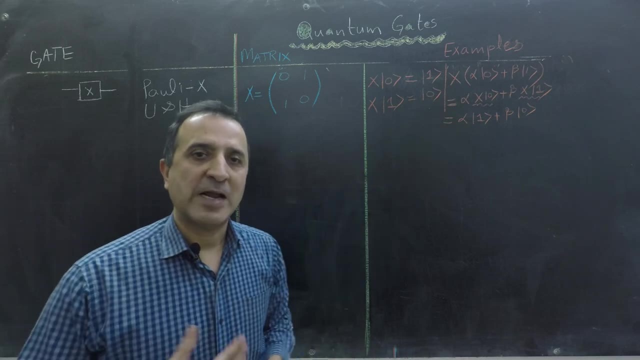 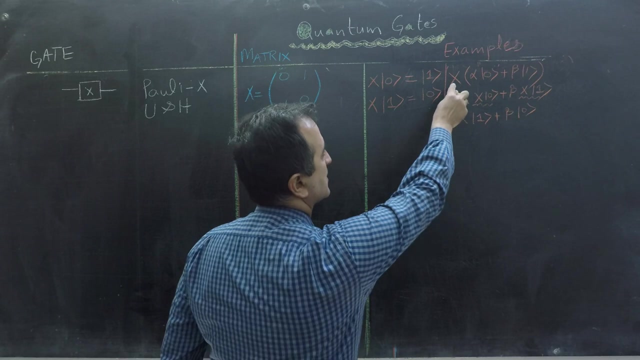 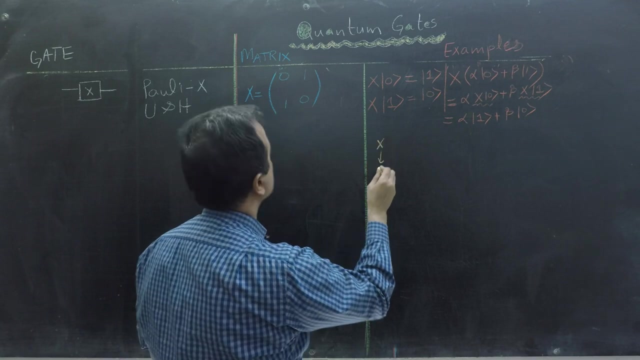 and how to apply it on any superposition. Before exploring another quantum gate, let's verify this thing using matrix and vectors, so that our concepts are crystal clear. To verify this, I write x in a form of matrix, So this is my x. 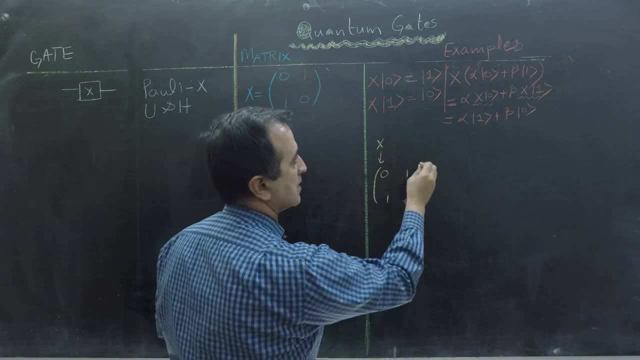 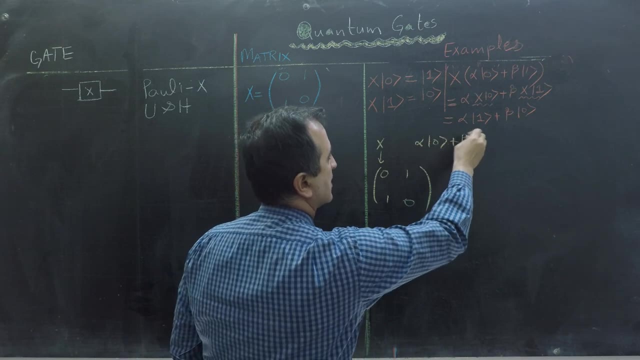 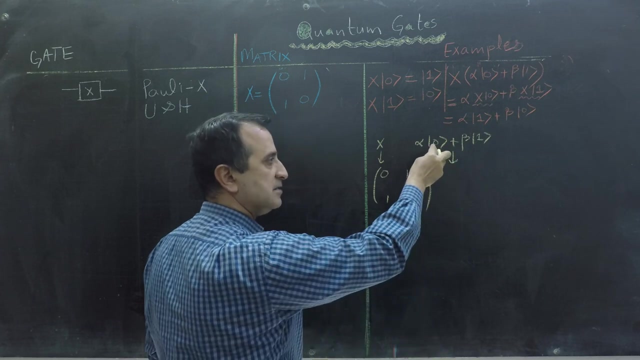 0, 1,, 1, 0.. And I write my vector, alpha- ket 0, plus beta, ket 1, in the form of vector, And because here at the 0th location I have alpha and at the first location I have beta, 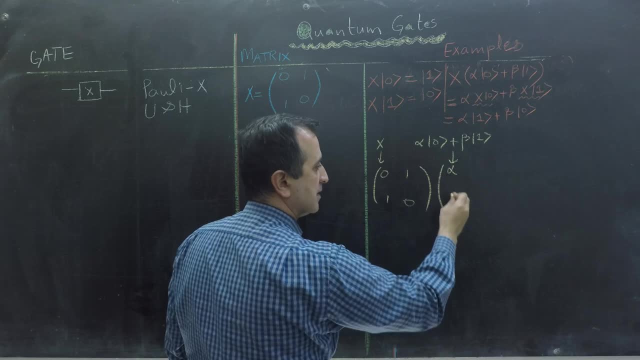 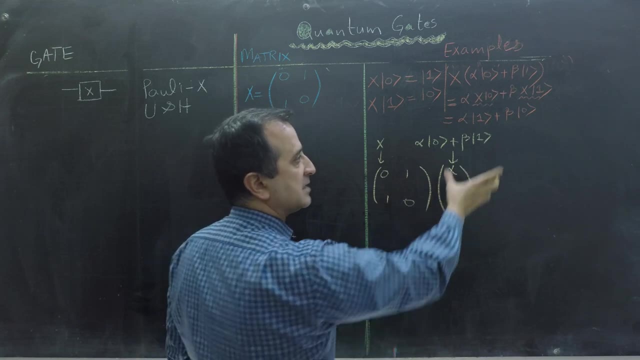 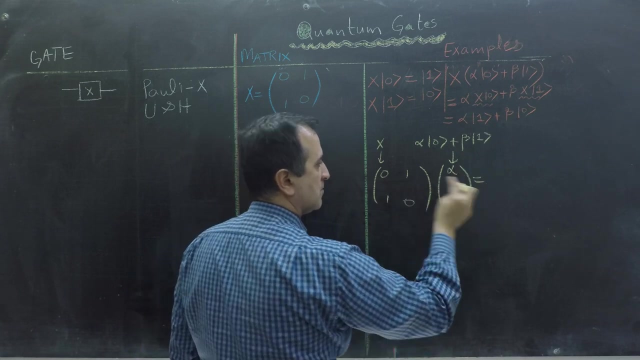 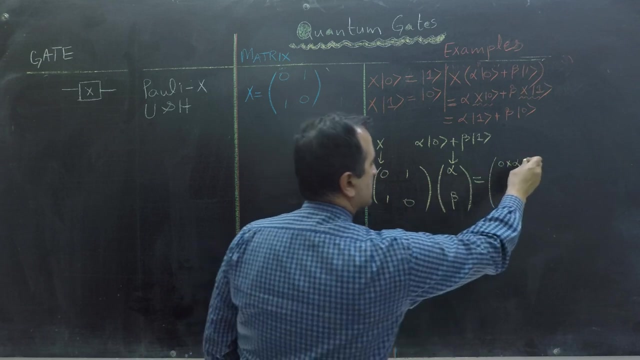 so my vector will be alpha- beta. Now I multiply this matrix with this vector to see if I get the same result or not. I multiply first row with column, getting 0 times alpha- 0 times alpha plus 1 times beta- 1 times beta. 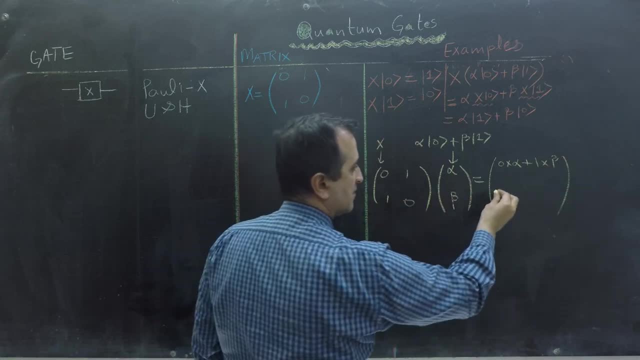 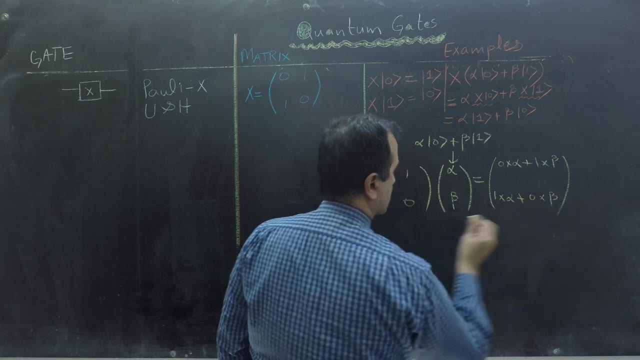 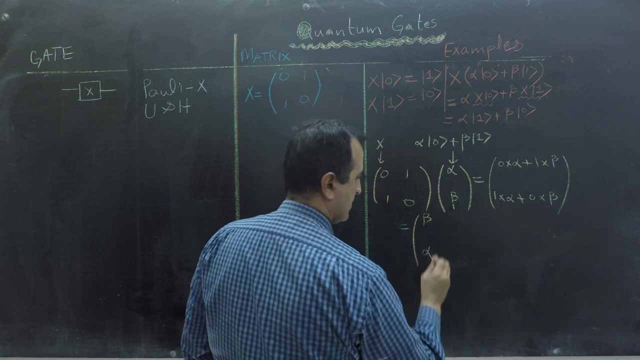 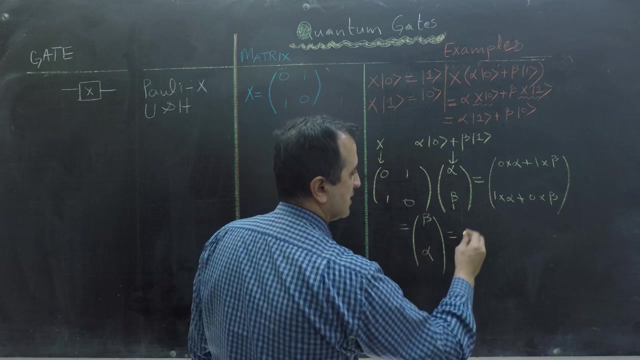 And here I will get 1 times alpha, 1 times alpha plus 0 times beta, 0 times beta. And this simplifies to beta alpha. and because 0th location has beta, so I can write it as beta times ket 0. and because my first location has alpha. 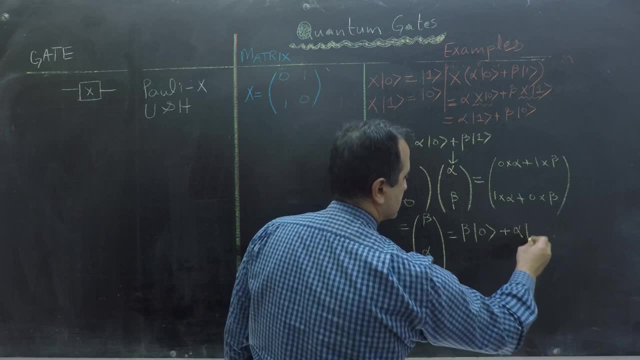 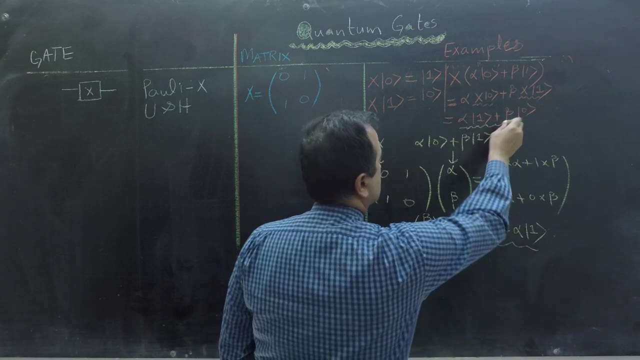 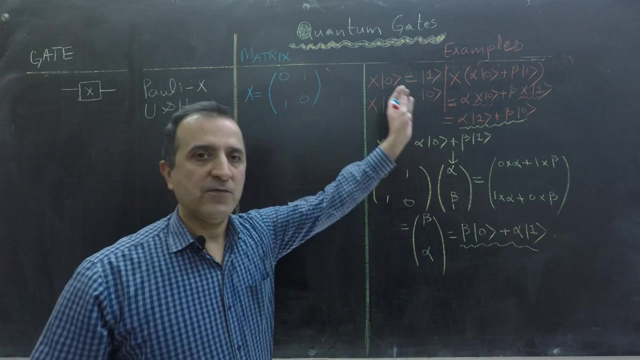 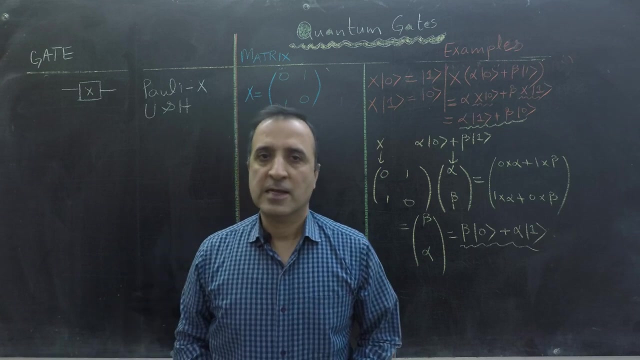 so I write it, plus alpha times, ket 1.. And you can see that this result and this result is exactly the same. So we have verified that this matrix behave exactly like we have written here. Now let's clear the board and then we will talk about. 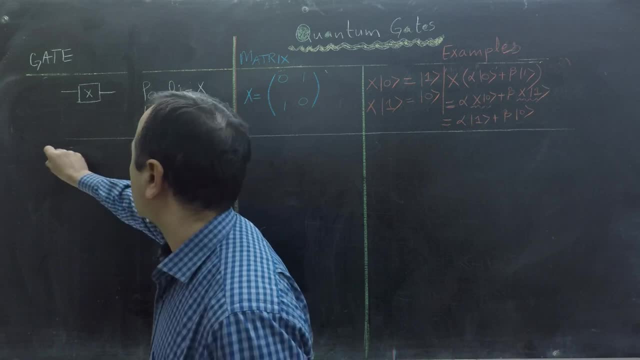 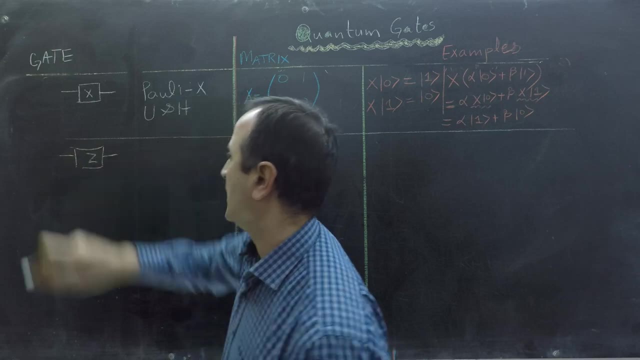 polyz gate. Polyz gate is also a single qubit gate, So it takes a single qubit as input. So it takes a single qubit as input. So it takes a single qubit as input And produces a single qubit output. 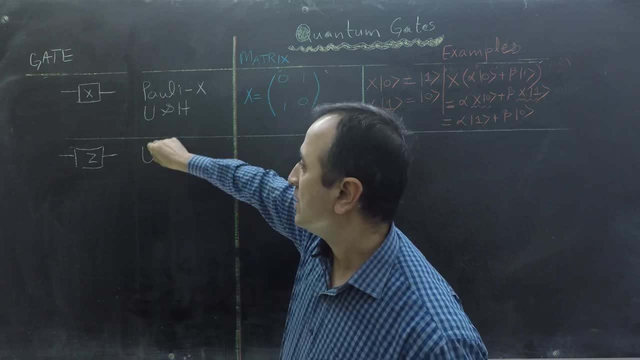 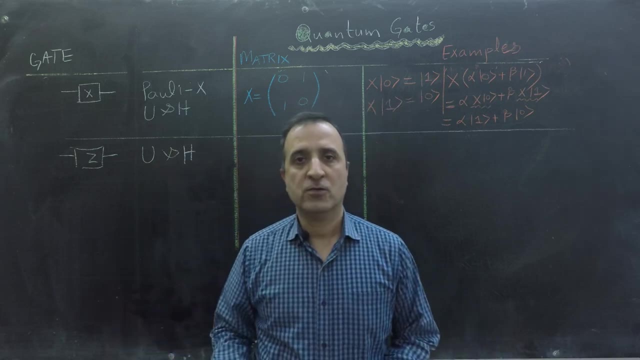 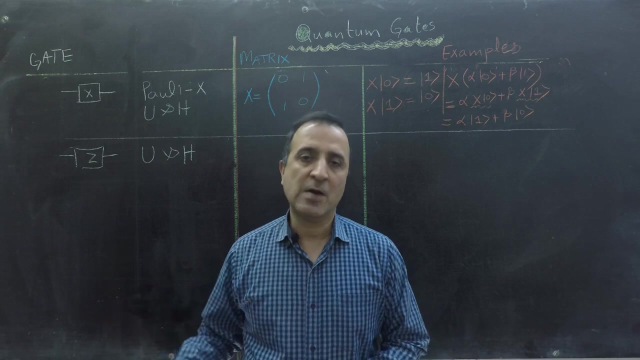 And it is also a unitary as well as a Hermitian gate. That means it is inverse of itself. So if I apply two polyz gates in sequence, they will cancel each other effect and my input will become equal to my output. Let's write the matrix of: 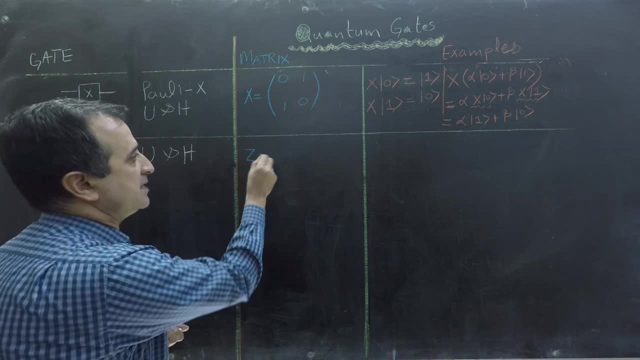 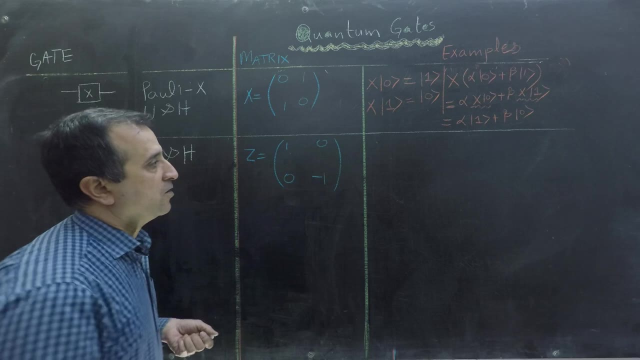 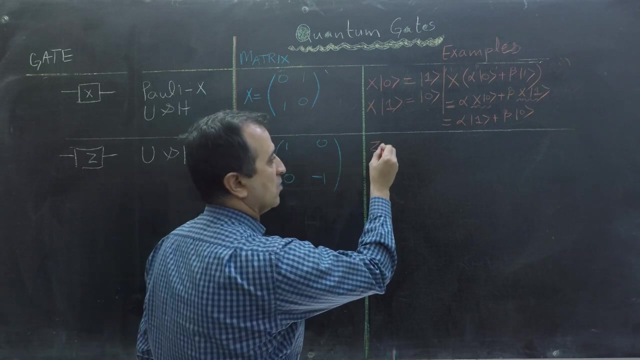 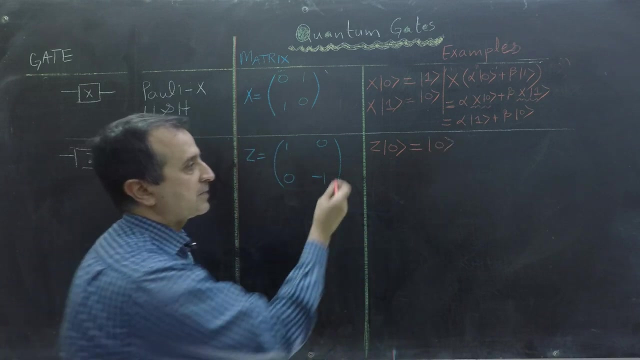 polyz gate. So the matrix of my z gate is Now let's see what is the effect of this matrix. If I apply polyz gate on ket 0, my answer remains ket 0. It does not change. And if I apply polyz gate? 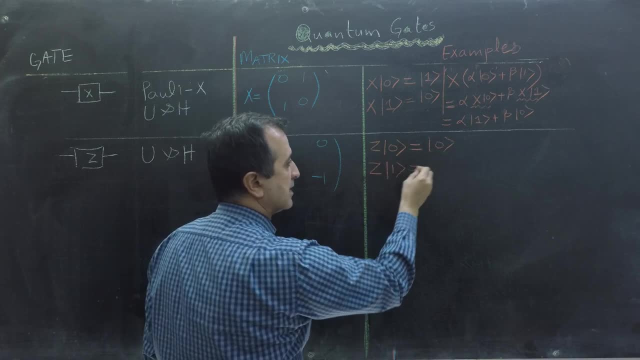 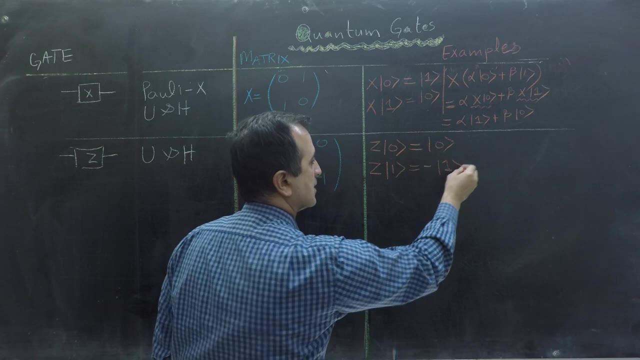 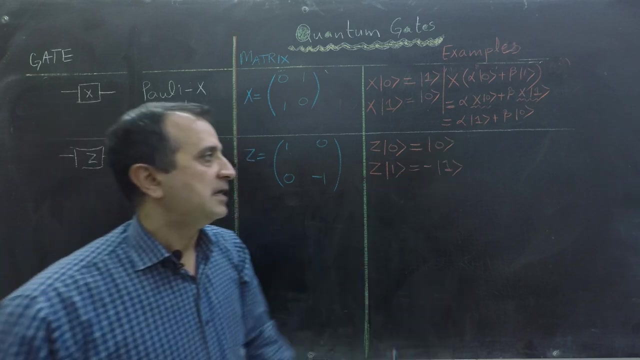 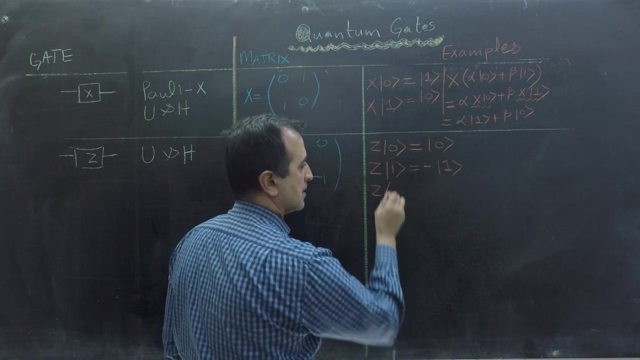 on ket 1, then I get a phase, So my answer becomes minus ket 1.. We can also apply polyz gate on superposition. Let's say I apply polyz gate on superposition of alpha ket 0 plus beta ket 1.. 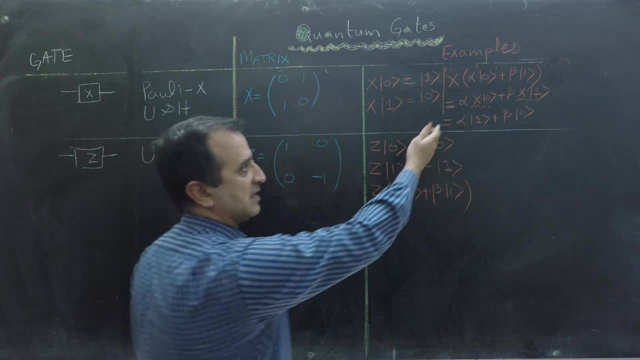 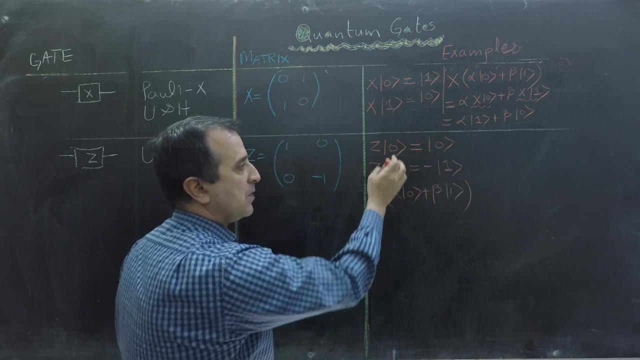 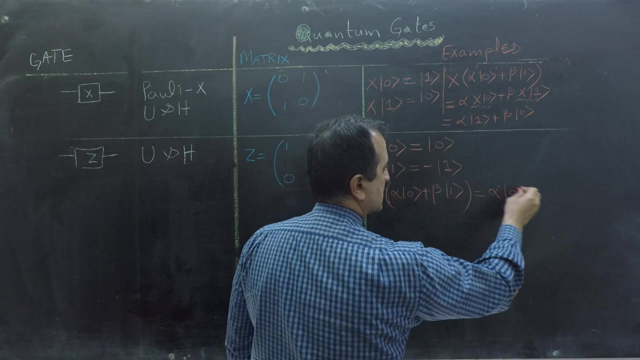 Then, because of the experience that we have with the x gate, we can quickly take z inside this summation and can apply z on ket 0 and ket 1, and our answer will be alpha. ket 0 remains the same, and here I will have a negative sign. 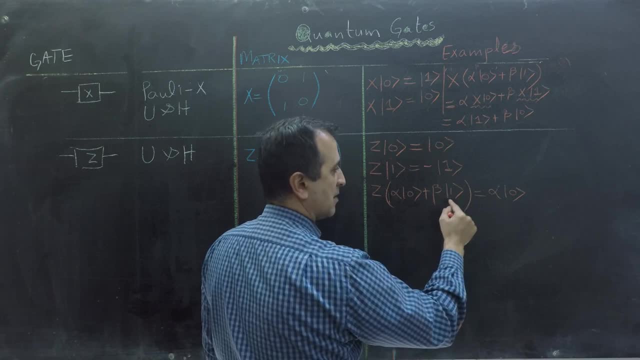 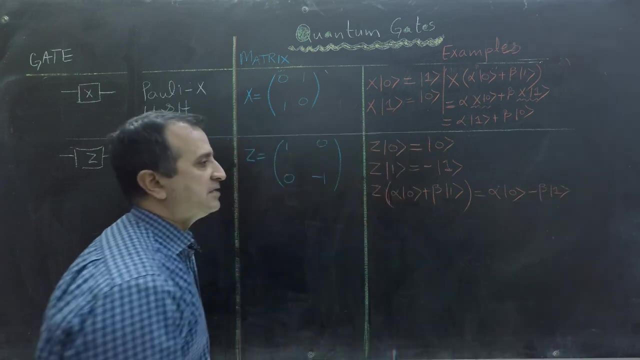 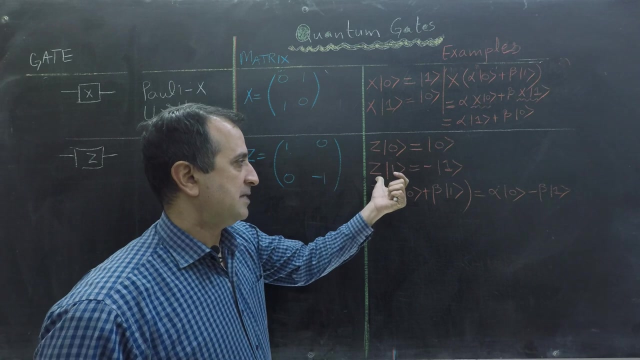 because ket 1 will become negative ket 1.. So I will get minus beta ket 1.. We can obviously verify any of this using this matrix. Let's verify this one. So what will be my result if I apply this matrix on vector ket 1.. 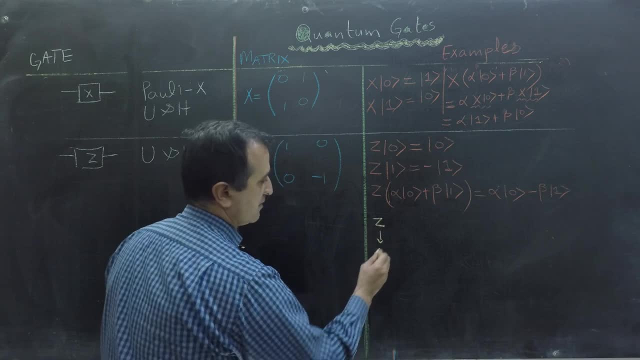 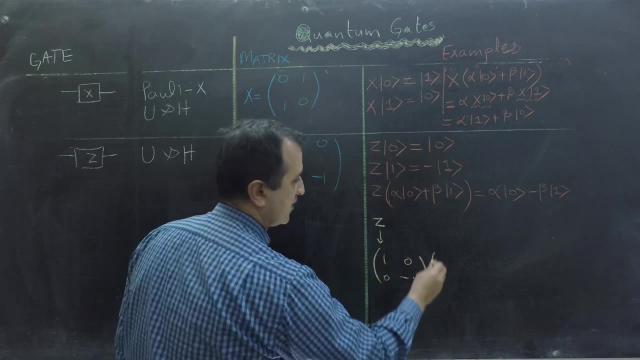 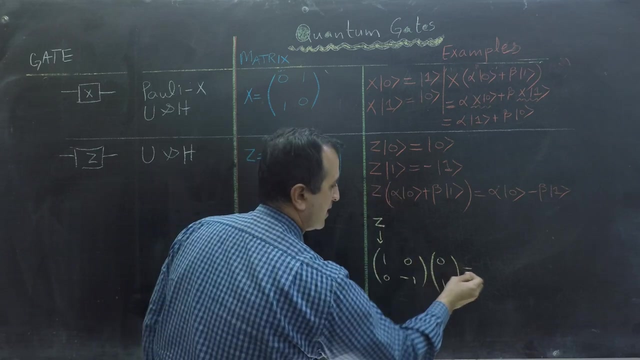 So here is my matrix, which is 1 0, 0 minus 1.. I apply this on vector ket 1.. That means my first location has 1 in it, Because this is ket 1.. And now I have to find my answer. 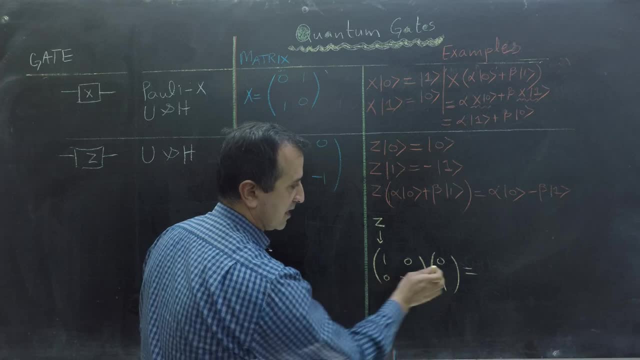 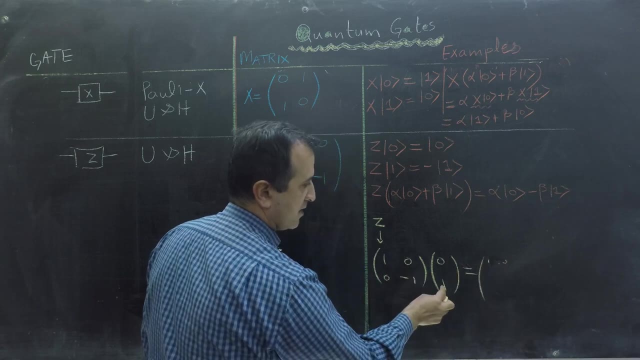 I multiply this row with this column: 1 times 0.. 1 times 0 is 0.. So I will have 0 here. And then 0 times 1 is also 0. So my answer will be 0.. Similarly, 0 times 0. 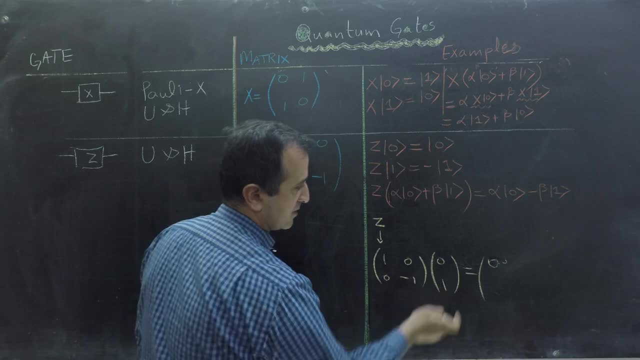 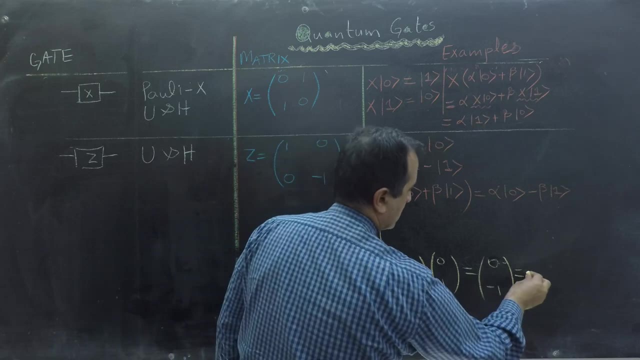 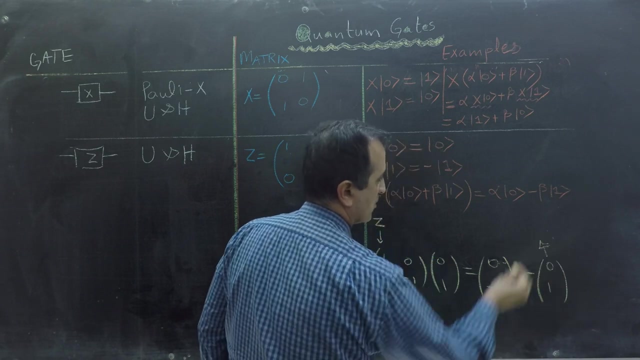 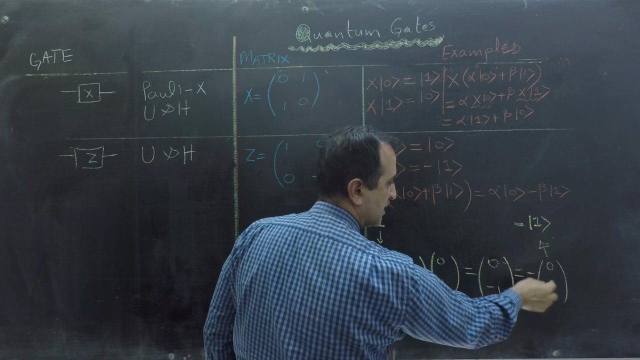 plus minus 1 times 1.. So I will have here minus 1.. And this simplifies to minus 0, 1.. And we know that we can write it in a ket notation of minus ket 1.. Because here at the first location I have 1.. 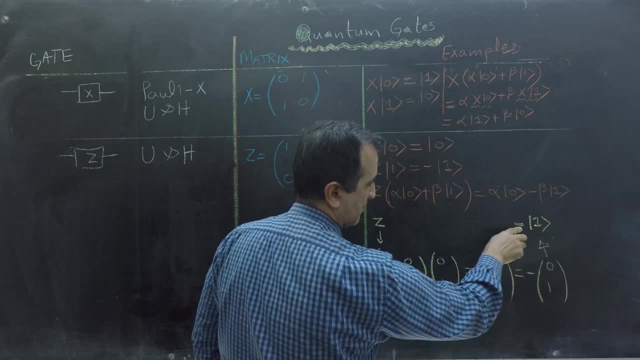 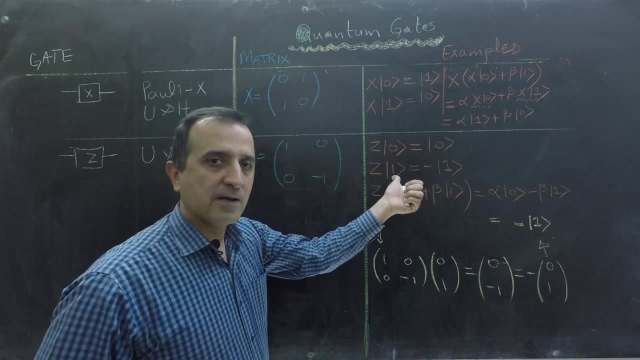 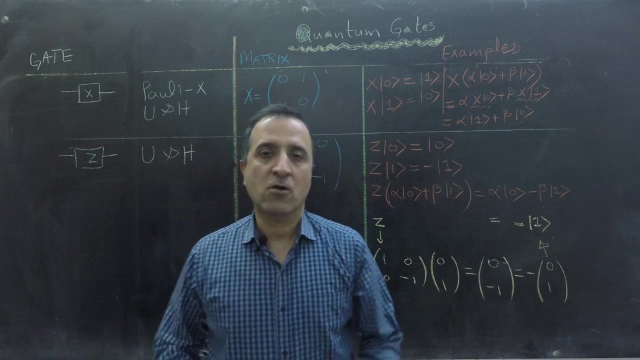 So this is ket 1. And minus is outside. So my answer is minus ket 1. And we have verified this. If I apply z gate on ket 1, my answer is minus ket 1.. Now let's look at another quantum gate. 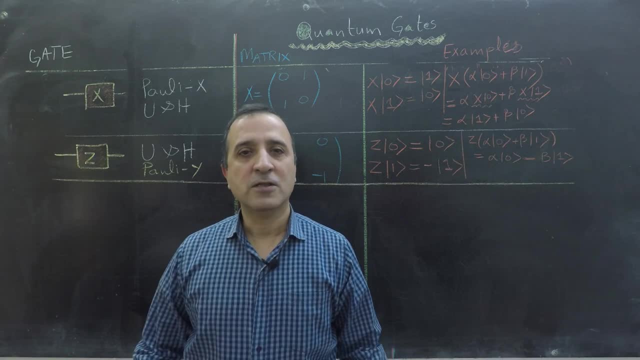 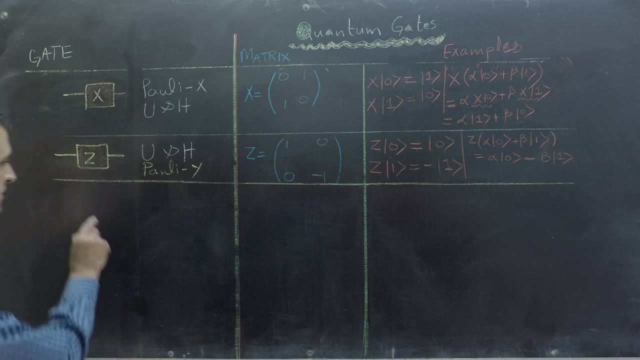 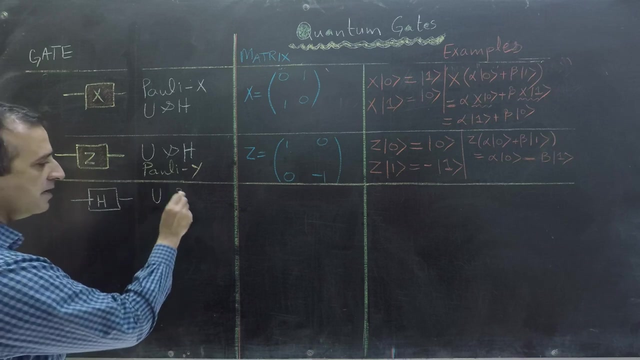 My favorite gate of all the gates is Hadamard gate. I even like its name, Hadamard. It is a single qubit gate which is also unitary and as well as Hermitian, And its name is Hadamard gate. 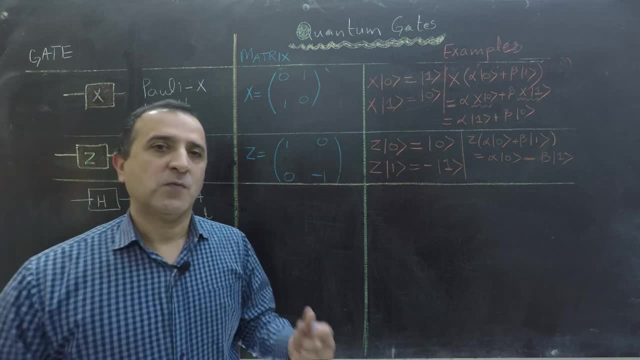 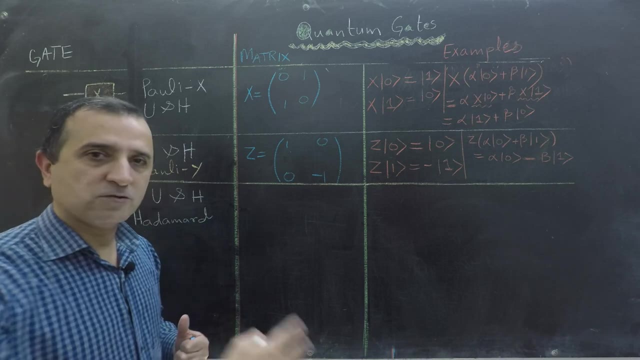 The reason I like this gate is because all quantum algorithm use this gate. So, to make it clear, I have made multiple videos about it, So you should go and watch those videos also. In this video I am going to just tell you this matrix and 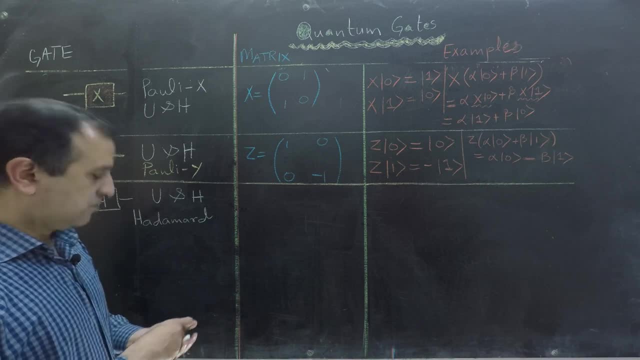 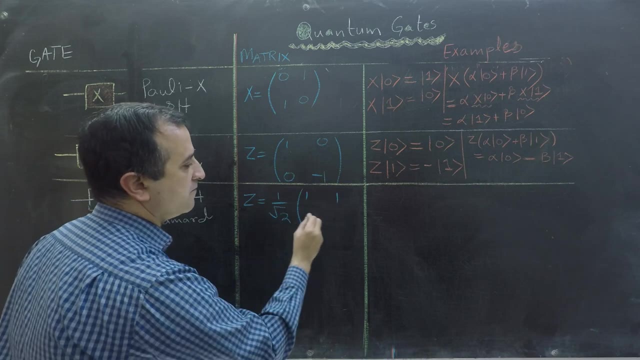 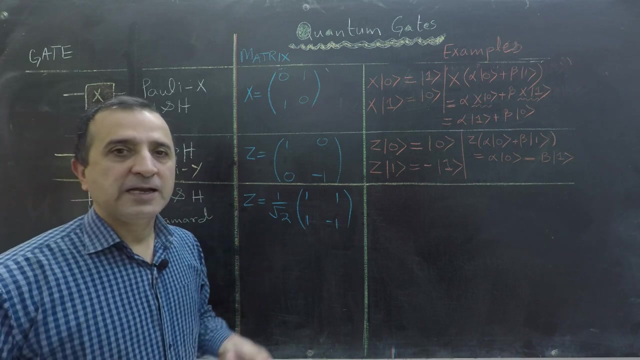 going to provide you a simple example. So the matrix of this gate is 1 over square root of 2.. 1, 1, 1 minus 1.. And this gate is used so often in all the circuits because it takes a pure state and 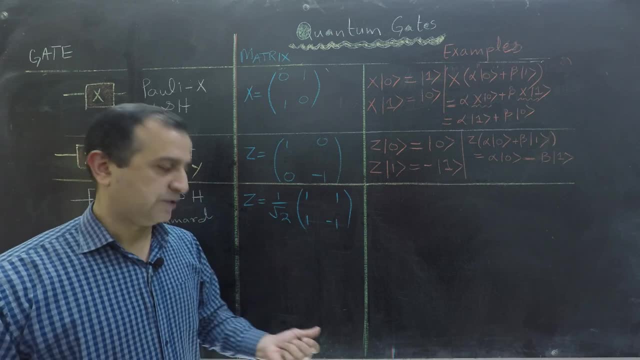 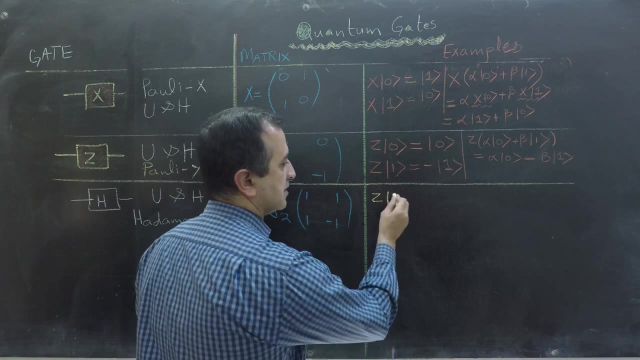 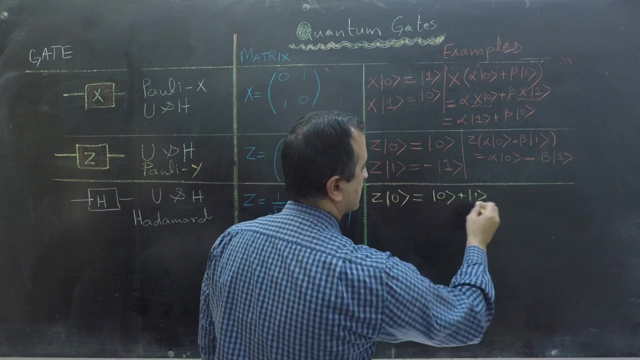 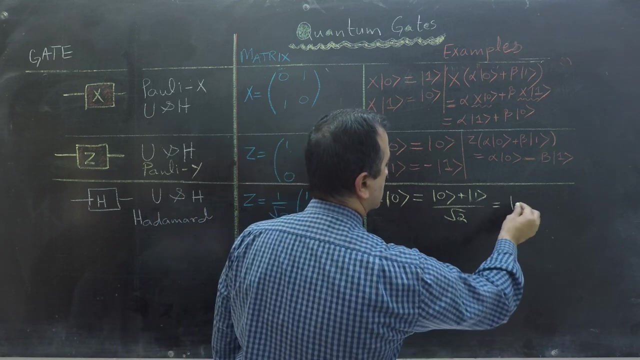 from that pure state, it creates an equal superposition. So if the input of this gate is ket 0, then the output will be ket 0 plus ket 1, divided by square root of 2. And this output is also known as ket plus. 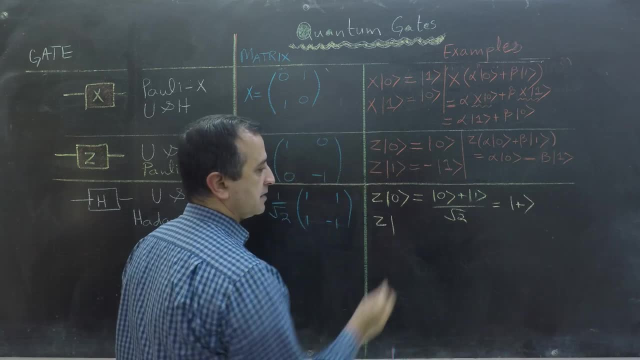 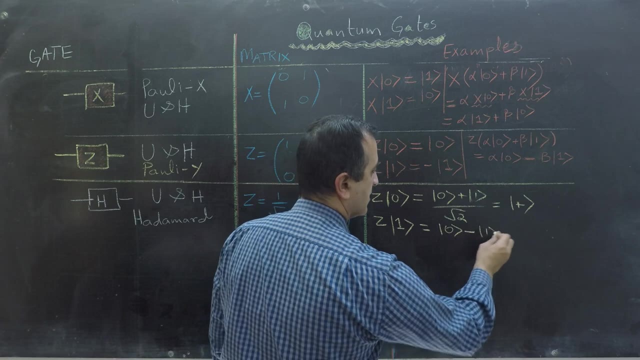 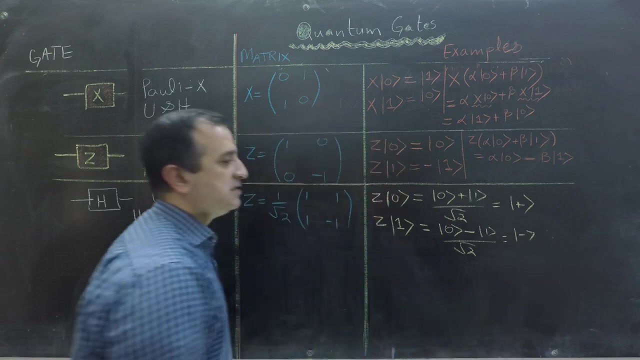 Similarly, if the input of this gate is ket 1, then the output will be ket 0 minus ket 1 divided by square root of 2. And this output is known as ket minus. Now, this gate is reversible, like all the quantum gates, because it is Hermitian. 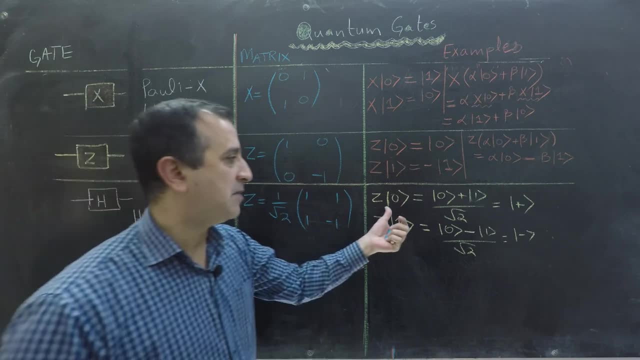 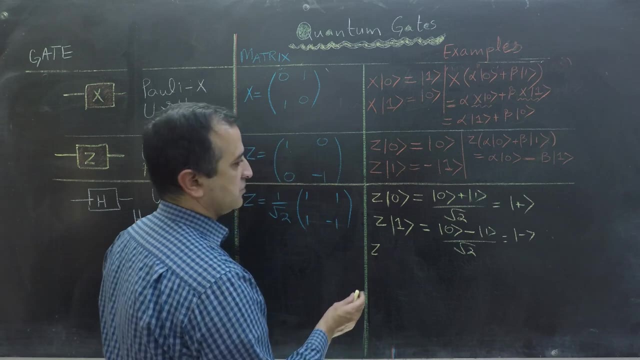 so it is reverse of itself. So if I put another Hadamard gate on this output, my result will be ket 0.. So if I say, oh, I should say Hadamard gate here, not Z gate, Why am I writing Z gate? 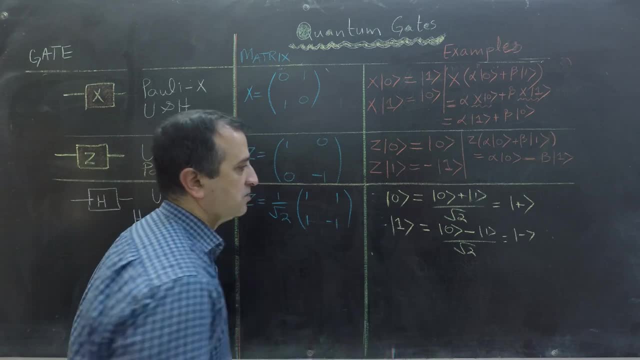 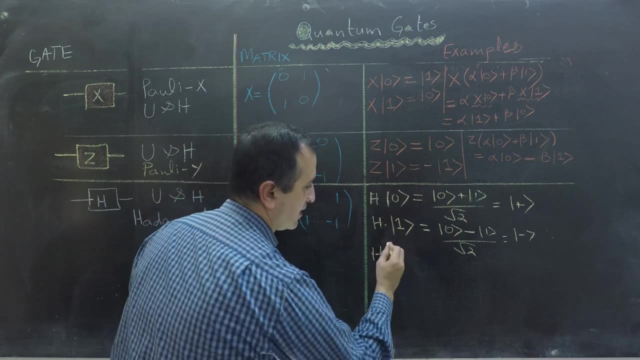 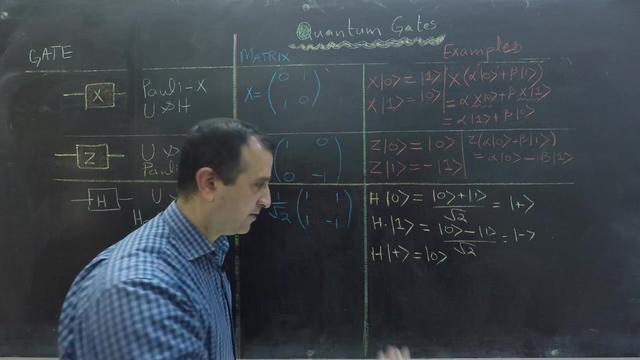 So Hadamard, Hadamard, Hadamard- Sorry, not Z gate, So Hadamard and Hadamard. So if I put Hadamard gate on input ket plus, then my answer will be ket 0, because this gate is reverse of itself. 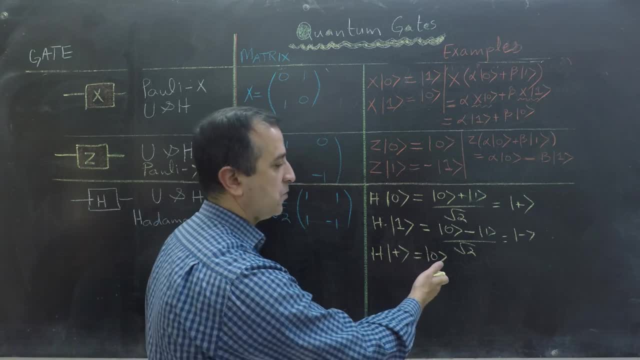 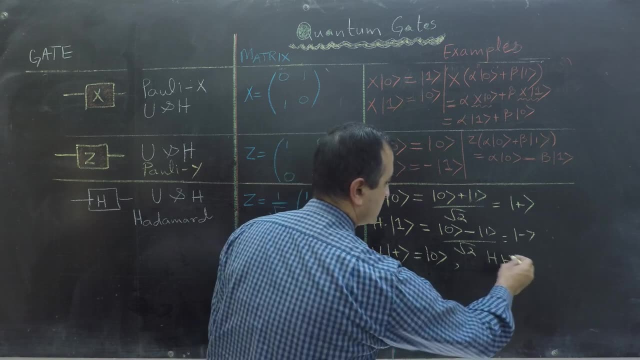 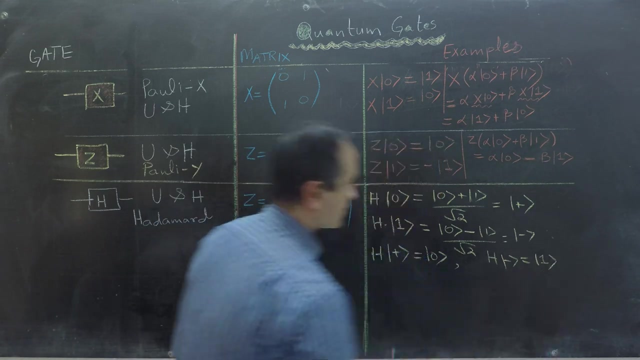 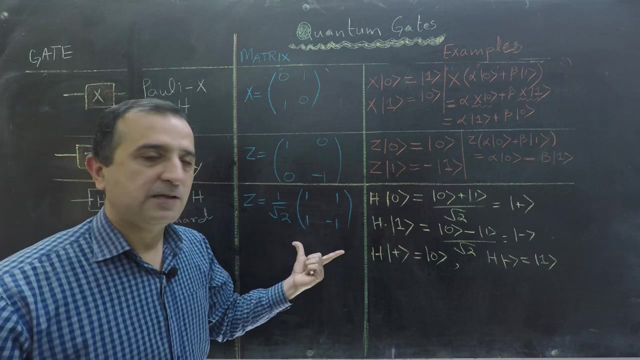 So it takes input ket plus and gives us output 0.. Similarly, if our input of this gate is ket minus, then our output will be guess ket 1.. We can obviously try this matrix to show that this matrix is working the way it is supposed to work. 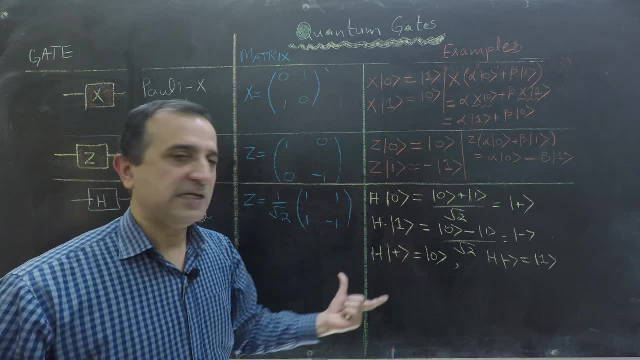 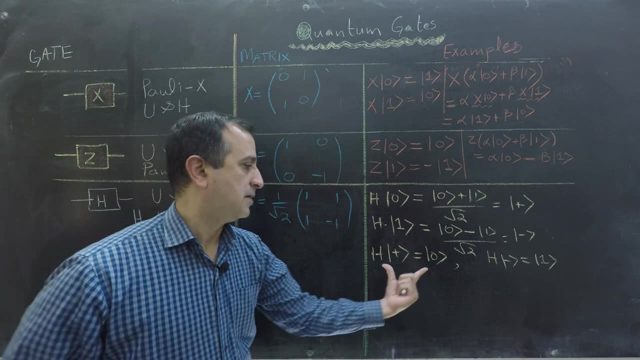 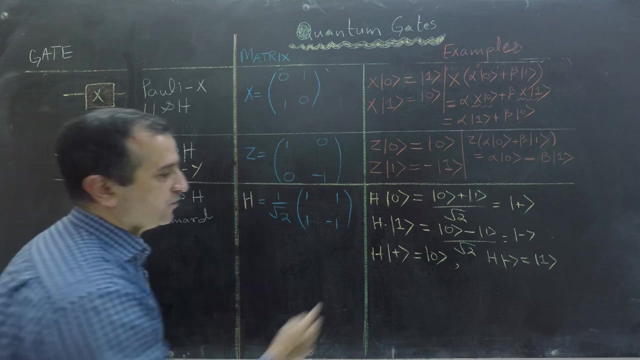 on any of those inputs and outputs and see if the result is exactly like we claim. So let's try, maybe this one. So I take my once again. here should be H not Z. So once again I try Hadamard gate on ket plus. So this is my. 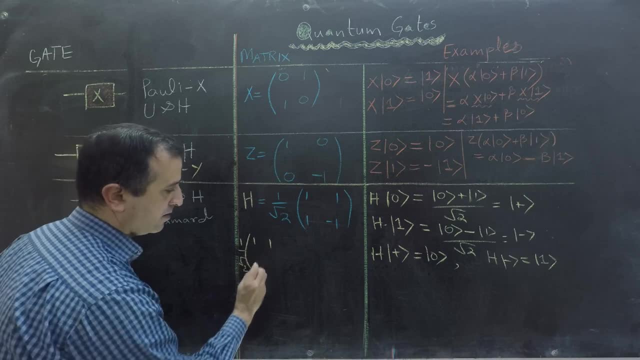 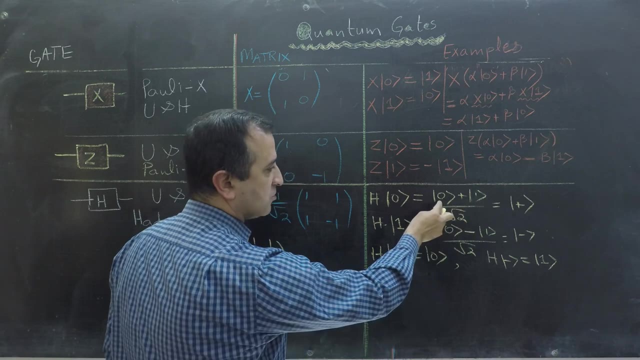 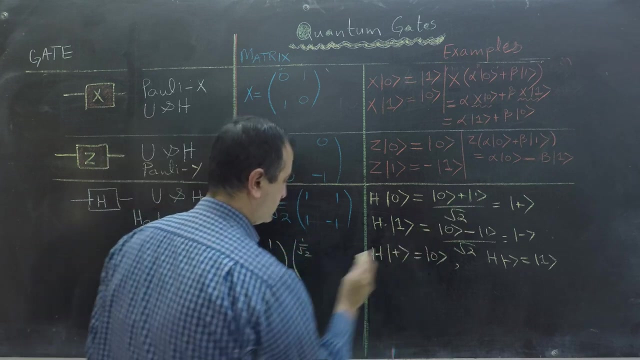 Hadamard gate on ket plus, and ket plus is defined as ket 0 plus ket 1 divided by square root of 2.. At the 0th location we have 1 over square root of 2 and at the first location we also have 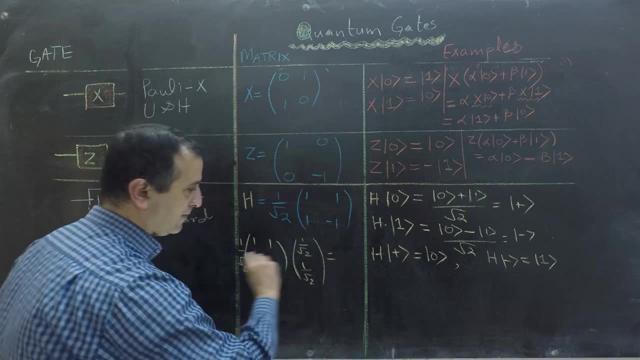 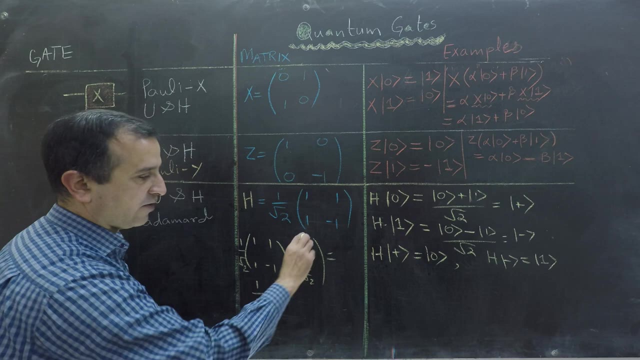 1 over square root of 2 and if we multiply our rows and columns we are going to get 1 over 2 outside, because I can take this 1 over square root of 2 also common. So this 1 over square root of 2 and this 1 over square root of 2. 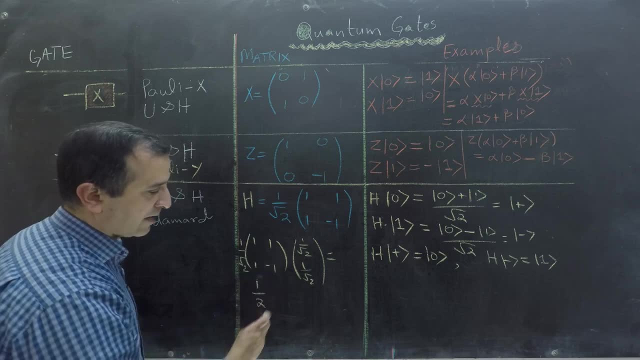 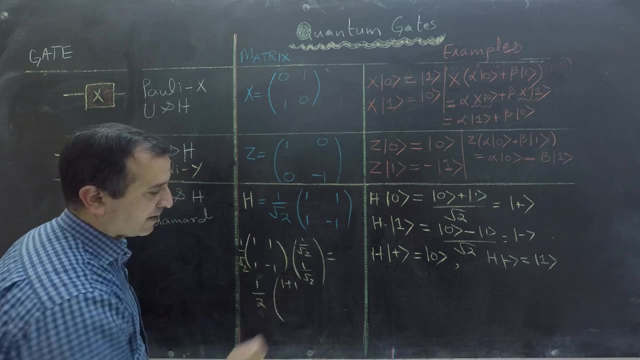 multiplies to become 1 over 2, and inside I will get 1 times 1 plus 1 times 1.. So it will be 1 plus 1.. Here and in this case, I will have 1 times 1 minus 1 times 1.. 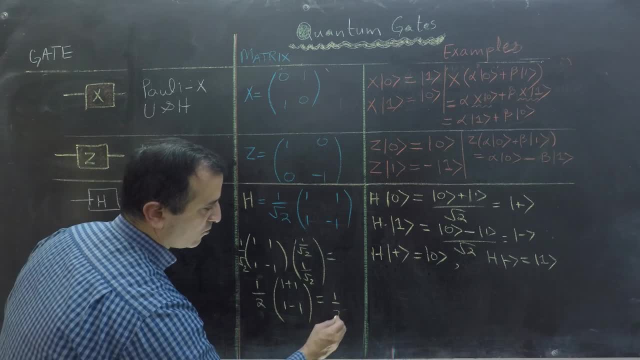 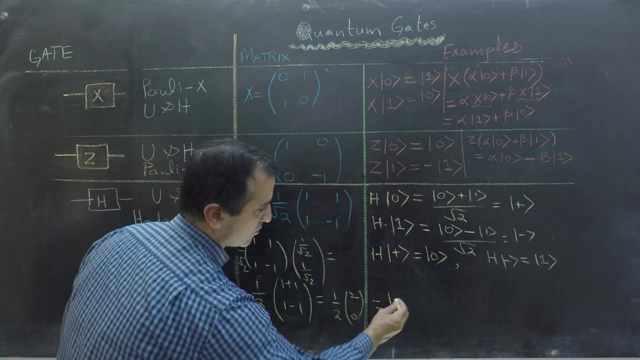 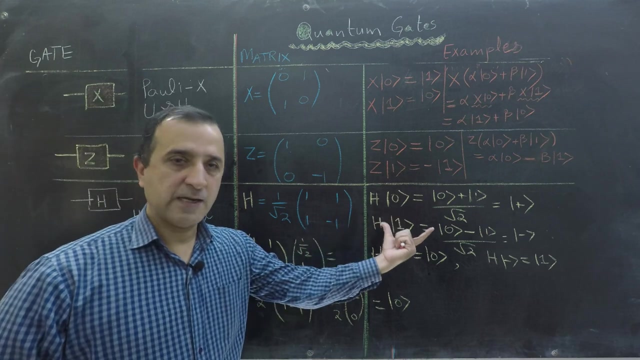 So my final result will be 1 over 2 and 2 over 0, which is equals to ket 0.. So, yes, this matrix works the way it is supposed to work. That means it takes a pure state and converts that pure state into: 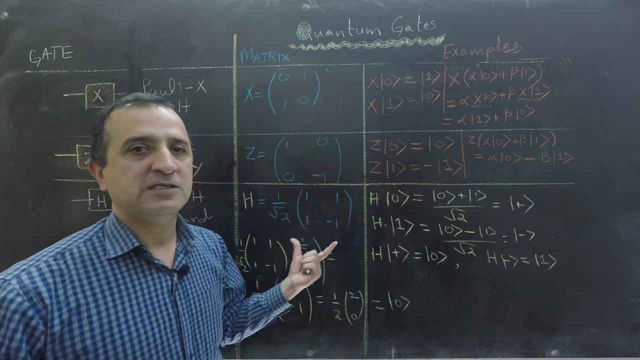 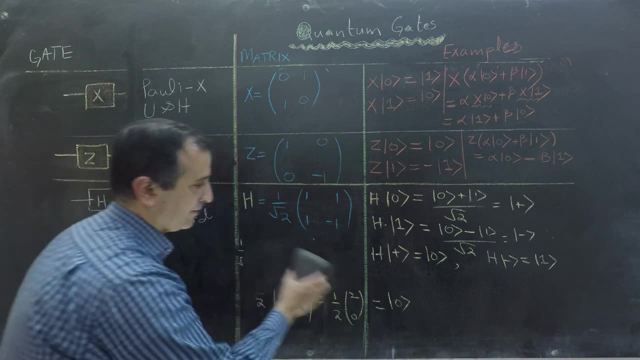 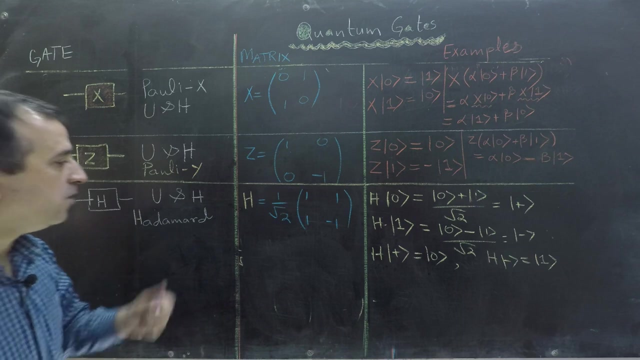 a superposition And we have multiple videos about it, because this gate is used extensively in many different ways. So please watch those videos also. Now you will be wondering that if all the gates are unitary and if all the gates are Hermitian all the time, 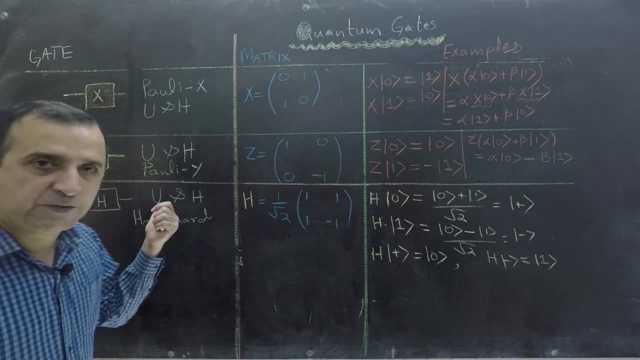 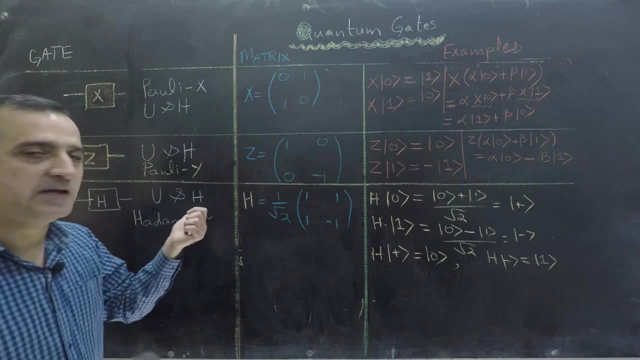 So the answer to this question is yes, all the gates must be unitary, as I have explained earlier, but all the gates don't have to be Hermitian, So they don't have to be inverse of themselves. So example of such a gate which is unitary: 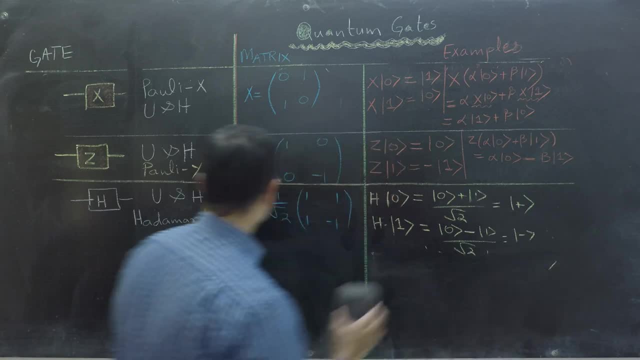 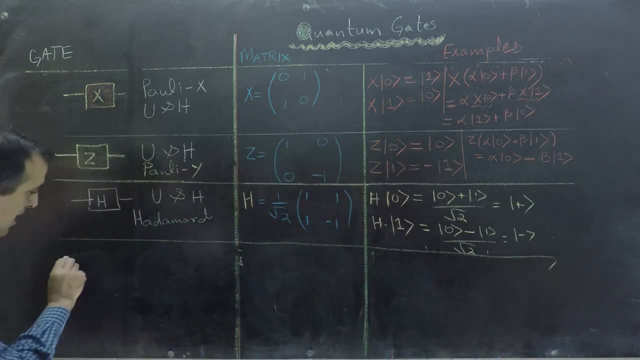 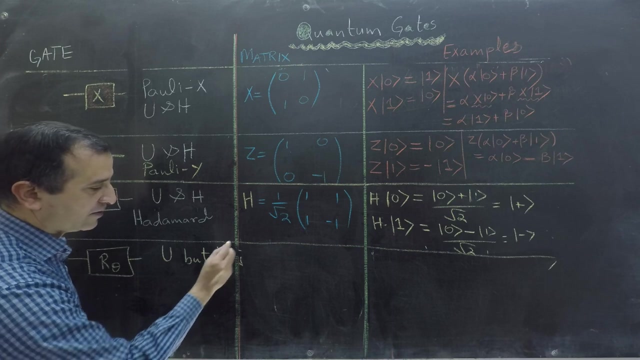 but not Hermitian, is rotation gate. So this is our R, theta or rotation gate. This is unitary gate. like all the quantum gates must be unitary but not Hermitian. So this gate is not reverse of itself. If you have, 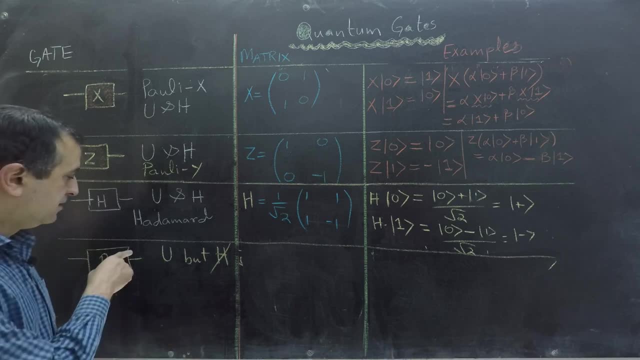 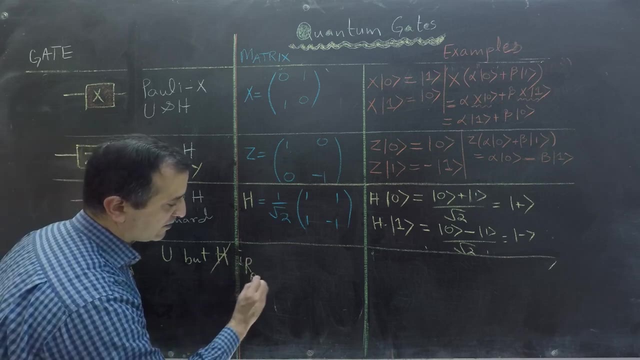 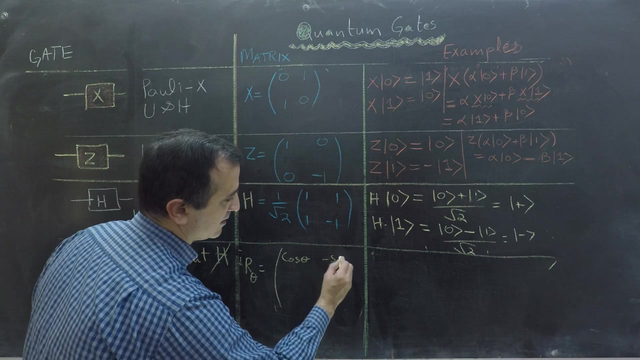 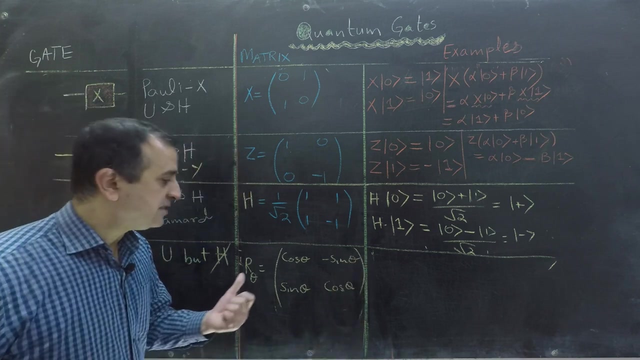 to find reverse of this gate you have to take conjugate transpose of this matrix. then you can get reverse of this gate. So R theta is rotation into dimension and this is equal to cos theta minus sine theta. sine theta, cos theta. So this matrix is: 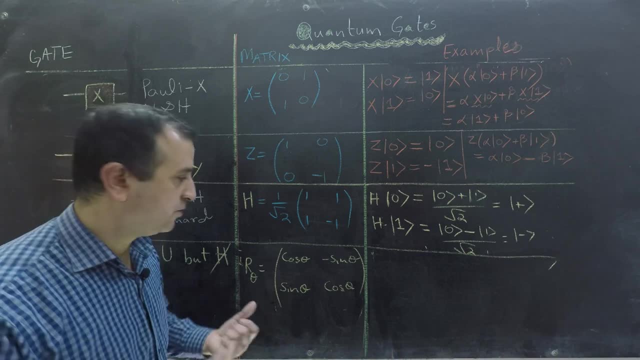 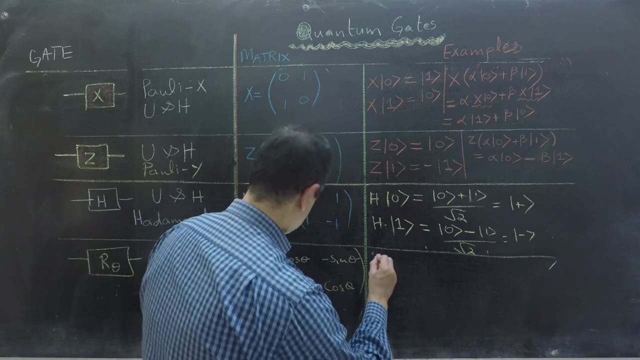 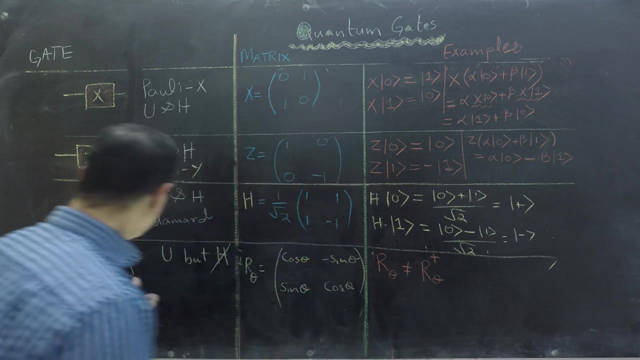 not Hermitian, because if I take transpose conjugate of this matrix I don't get the same matrix. So in this case my R theta is not equal to R theta transpose conjugate. But this matrix is unitary because if I take R theta 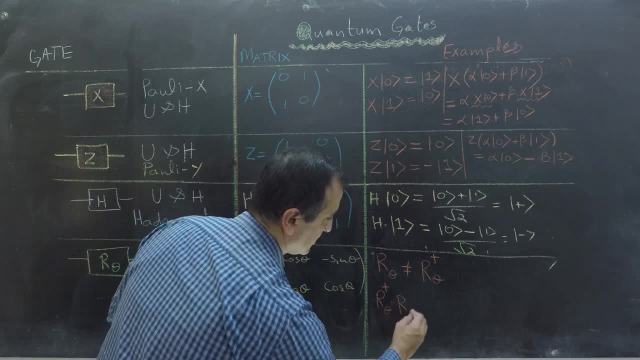 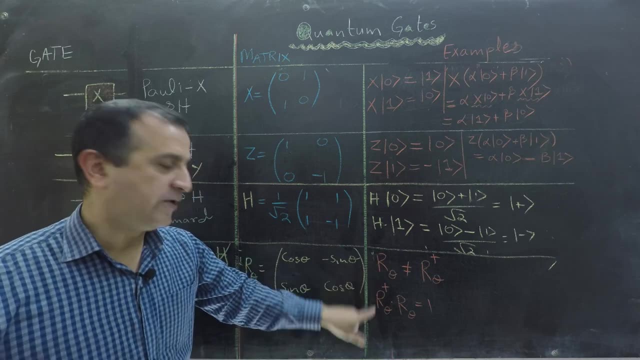 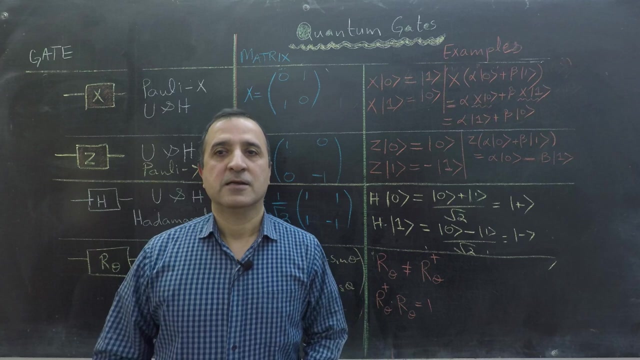 and take, transpose, conjugate and multiply with R theta, my answer is always equal to identity. So it will be an interesting quiz question to make you verify both of those things. Now let's look at the two qubits gate like control gates and swap gate and etc. 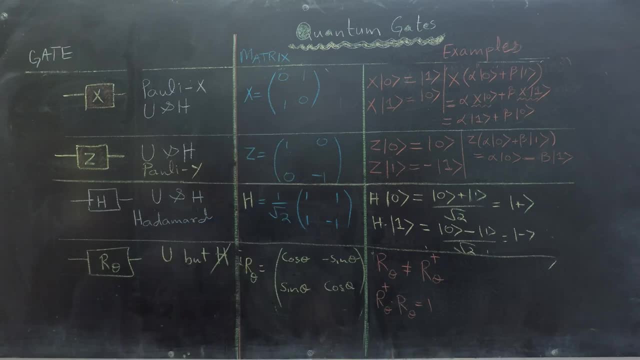 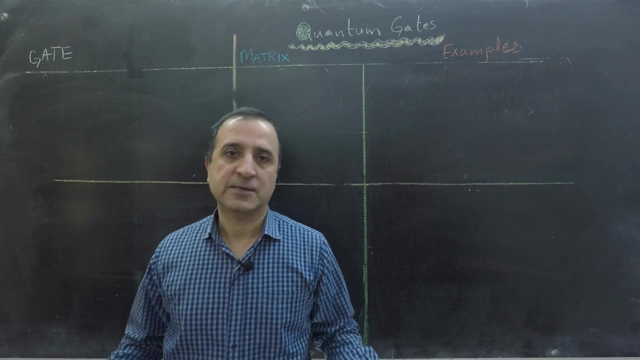 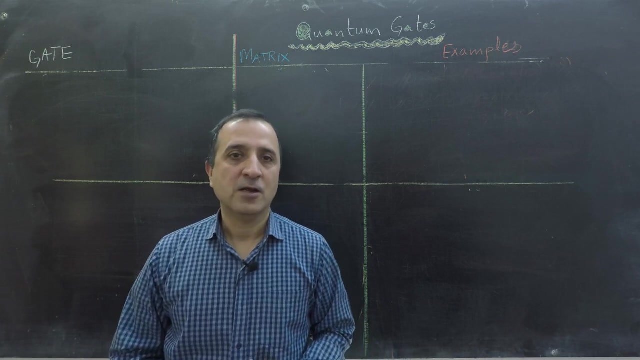 For that I must clear the board first. It is time to look at many two qubits gates. Now recall that we said that if we have a single qubit then we need 2 by 2 matrices as quantum gates, And if we have n qubits we need 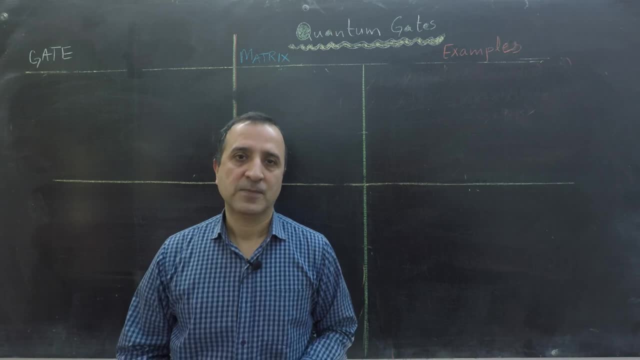 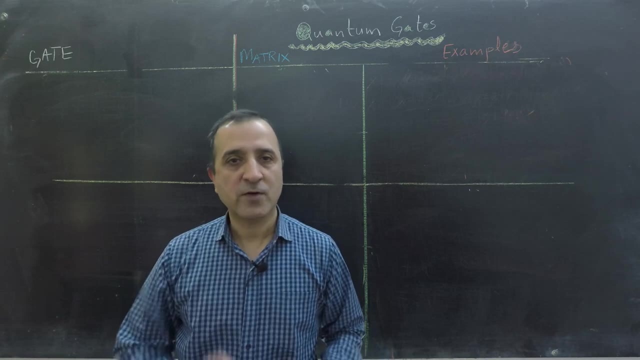 2 raised to power n, times 2 raised to power n matrices as quantum gates. What about 2 qubits? So if I have 2 qubits, then my matrices will be 4 by 4.. Now let's look at a swap gate that takes 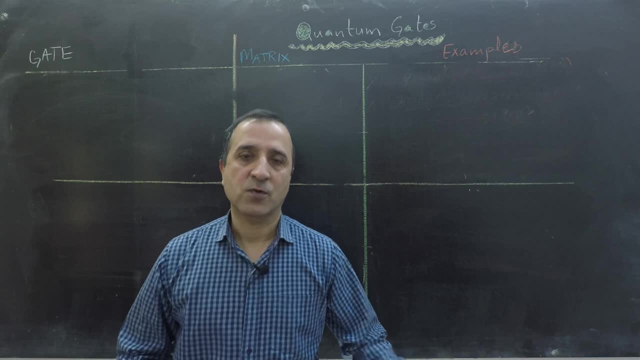 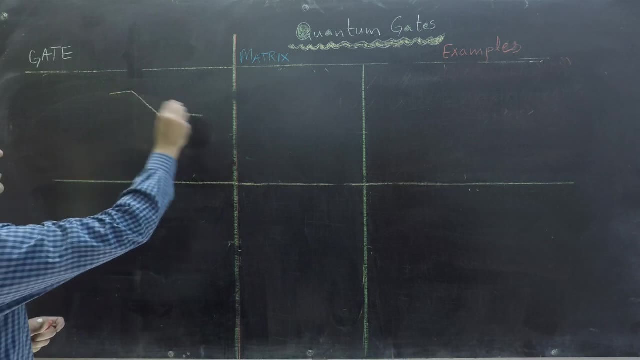 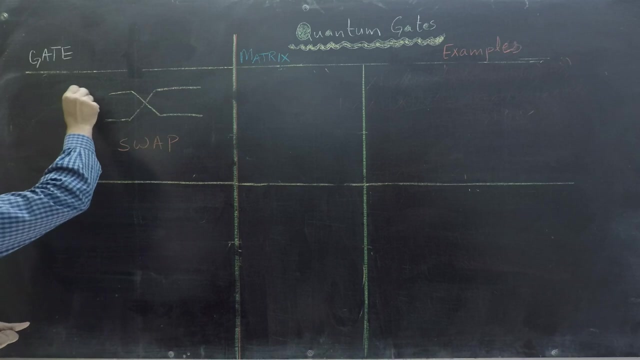 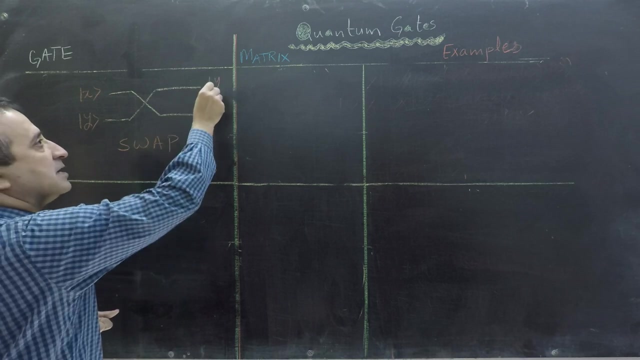 two inputs and then swap them at the output. So this is my swap gate And it takes two inputs and then it swaps those inputs. So if my input is x here and if my input is ket y here, then on the output my output will be. 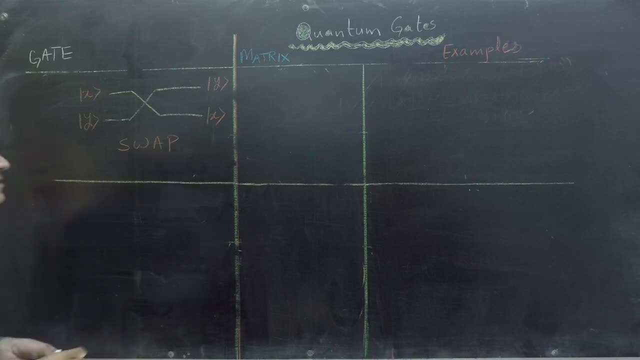 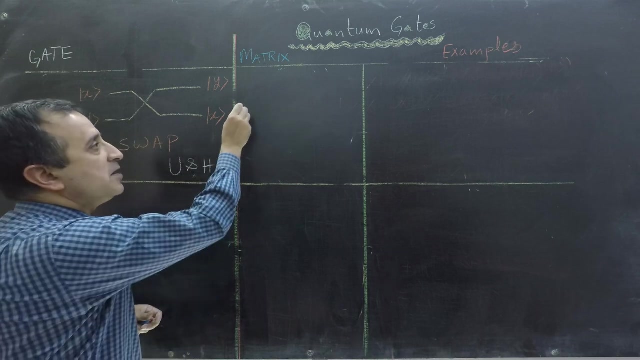 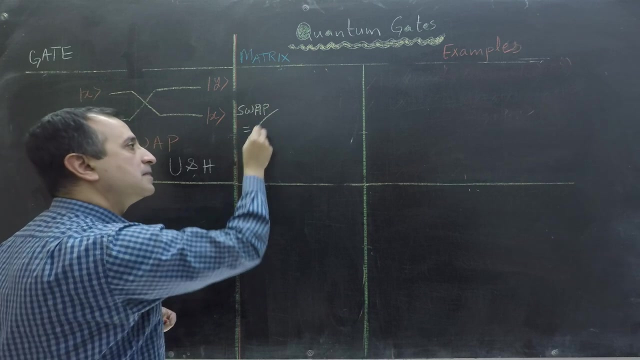 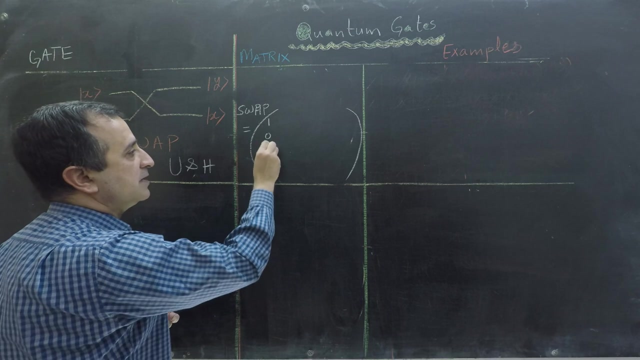 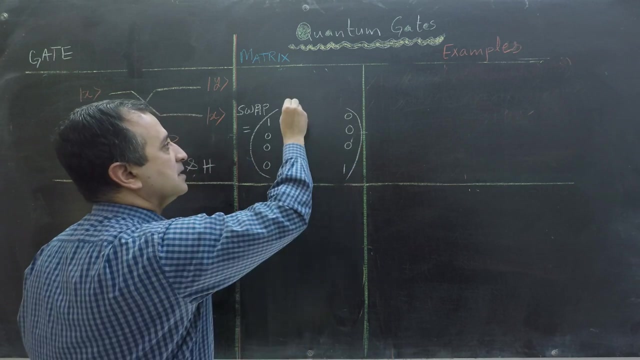 y and ket x. This gate is unitary and hermitian. The matrix of swap gate is as follows: There we have the first column of identity matrix and the last column of identity matrix, But the middle two columns are swapped with each other. 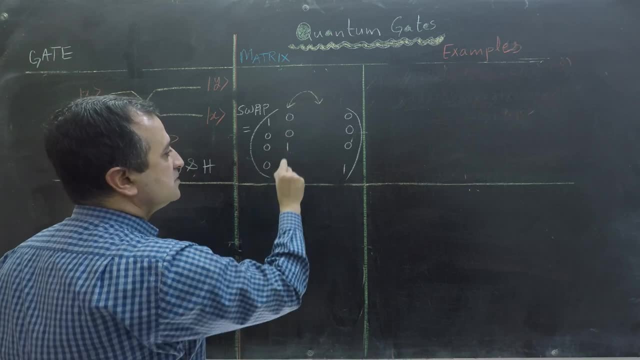 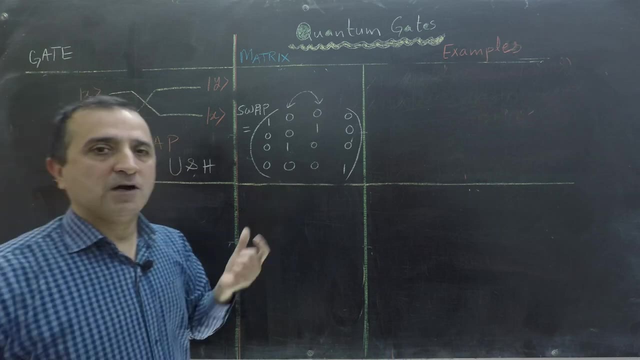 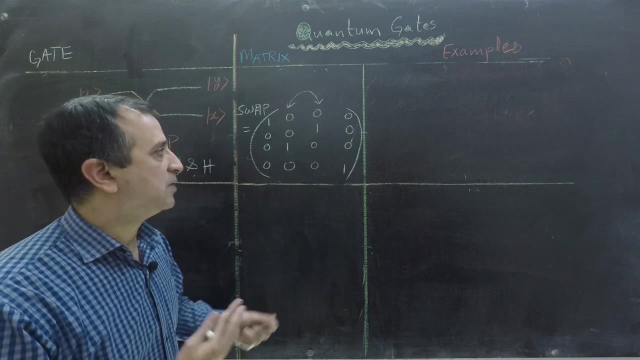 So here I will have 0 0 1 0, and here I will have 0 1 0, 0.. So these kind of matrices are also known as permutation matrices, which are basically identity matrix, but some rows and columns are swapped. 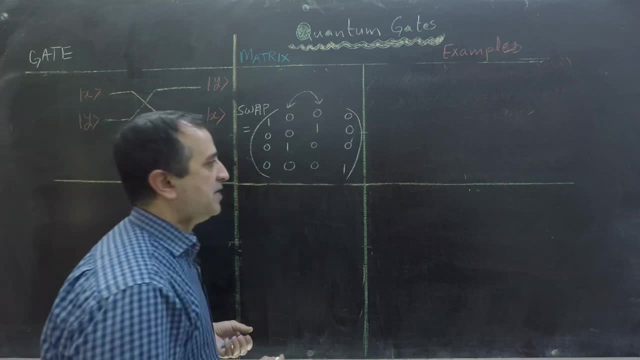 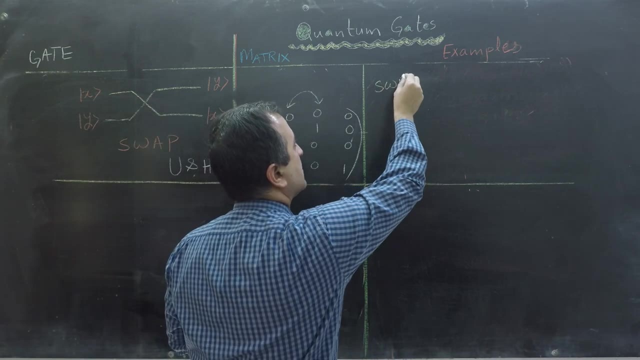 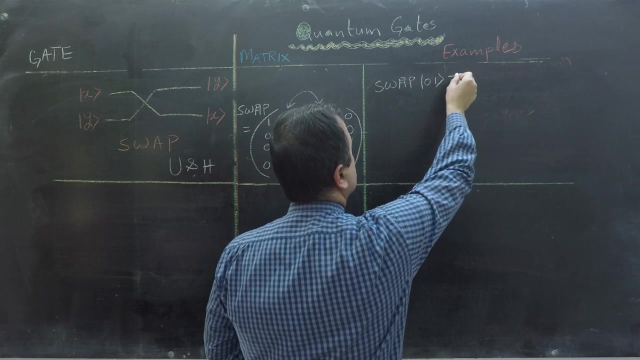 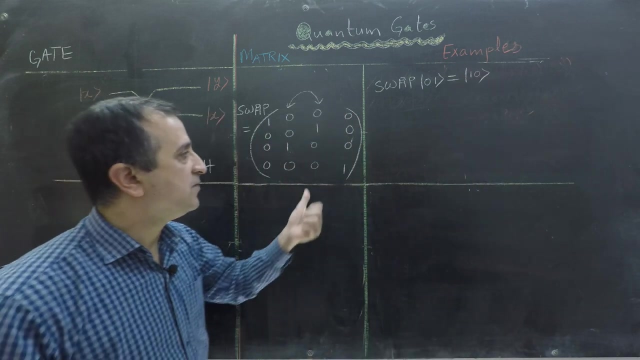 So we can test this matrix on some input to see if it is really swapping the inputs. Let's try this: that I give swap gate input of ket 0- 1, then our claim that our output will be 1: 0.. Now we verify that swap gate. 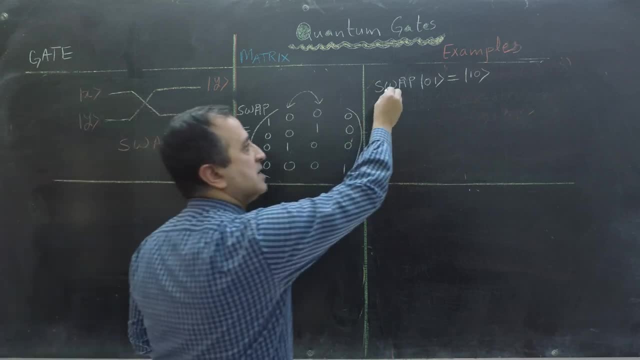 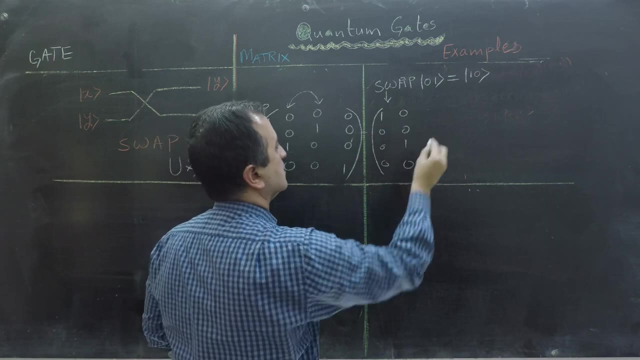 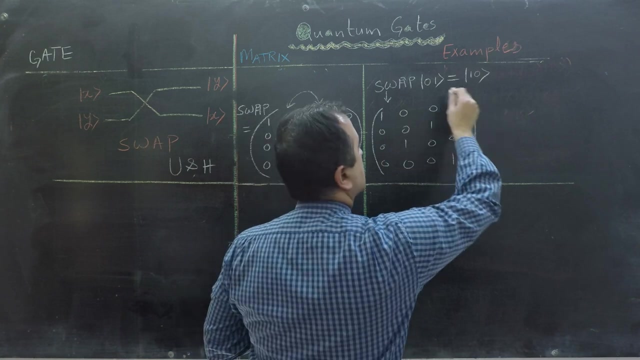 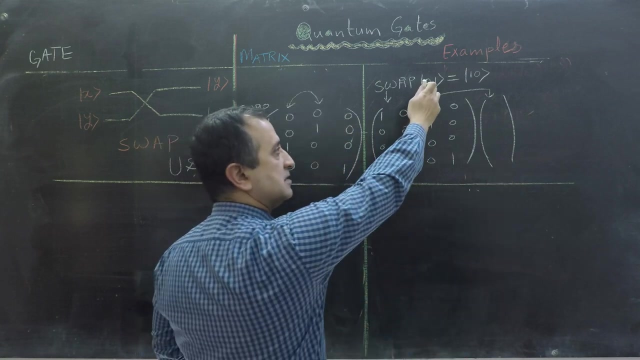 works this way, using this matrix. So here I plugged in my matrix And now I write my input here, which will be a 4D vector whose first location will have one in it. So this is my zeroth location, this is my first location. 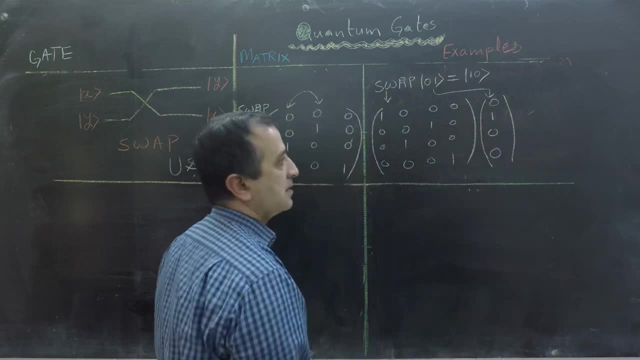 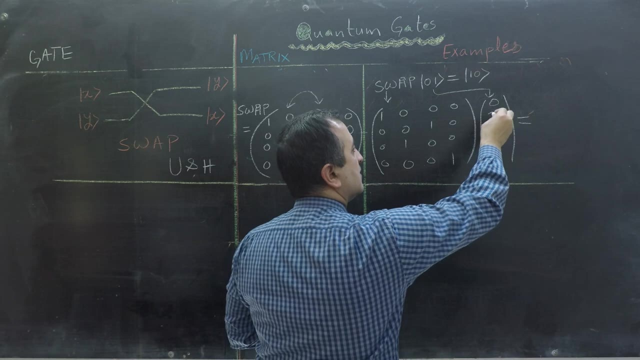 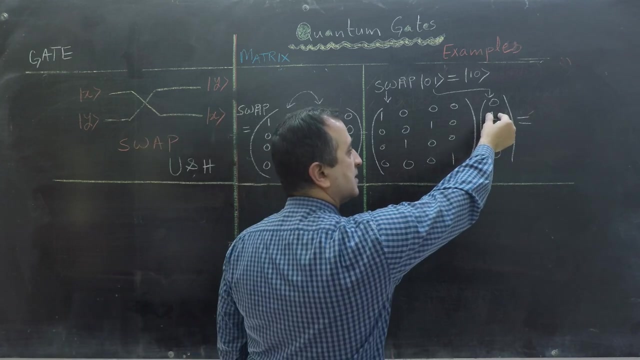 this is my second and this is my third location, And now I have to find the answer. A simple way to find answer is to write the first column, Because I have one at the first row of this vector, so my result will be first column. This is just a. 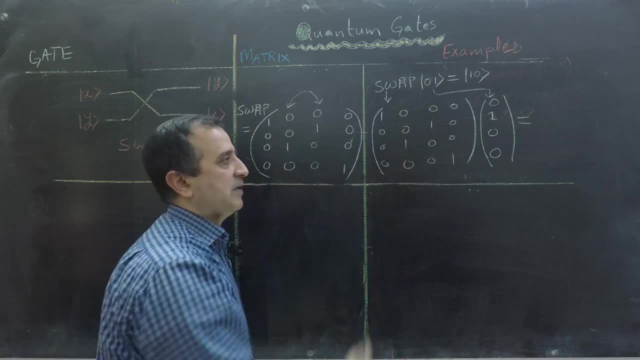 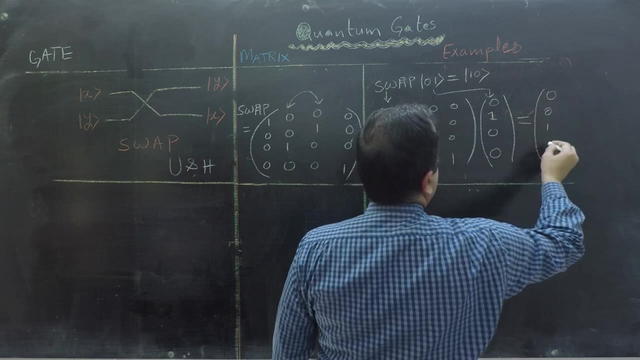 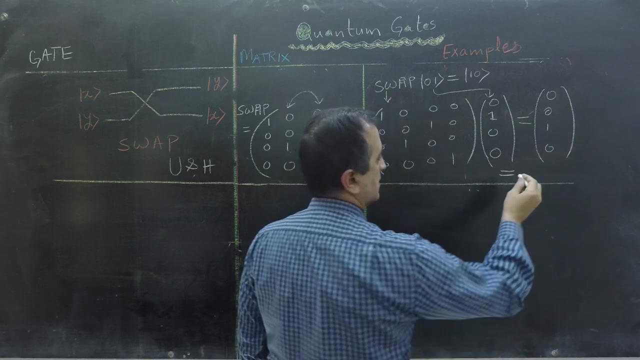 shortcut to find the result quickly. Or you can try to multiply this and the result will be anyway this column 0 0 1 0, and this is equals to 0 ket 1 0, because now my 1 is at the second location. 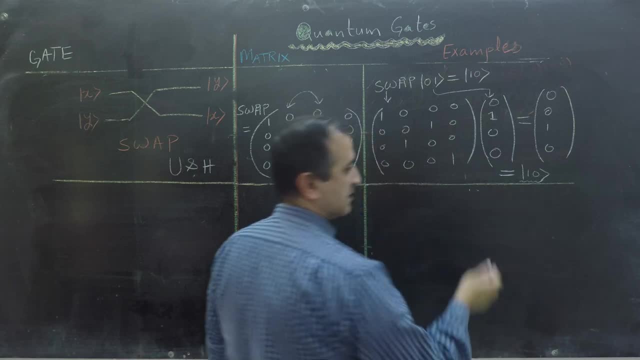 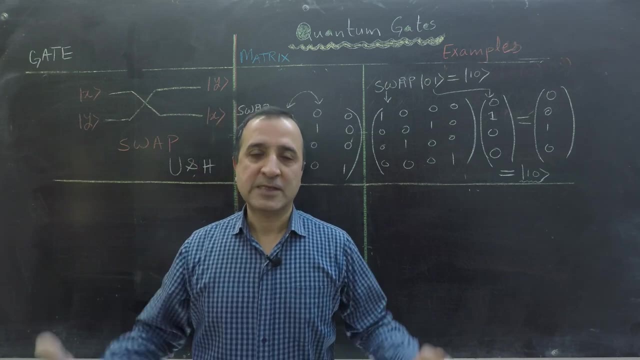 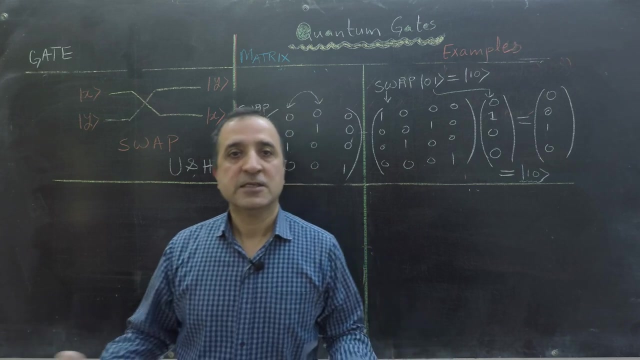 So my result will be ket 1- 0, which is ket 2.. There are some series of two qubits gates which are called as control gates. The one of those gate is c0 gate, But there are also control z gate, control x gate. 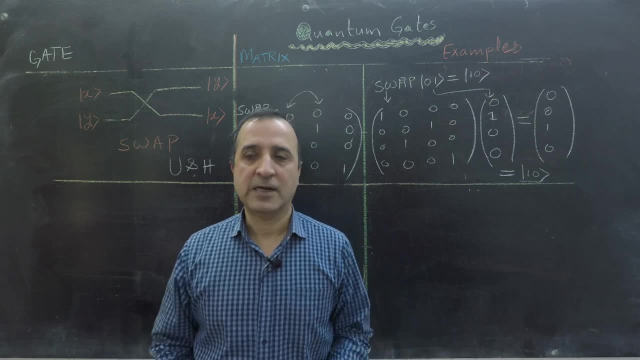 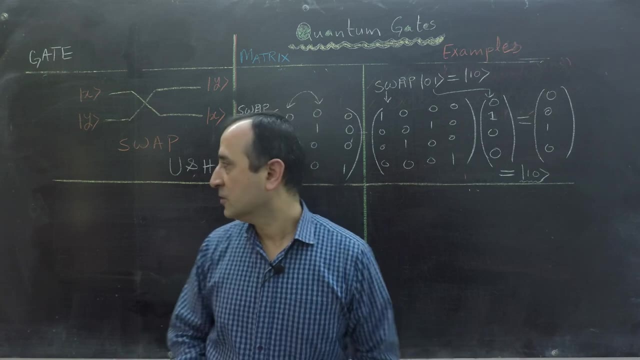 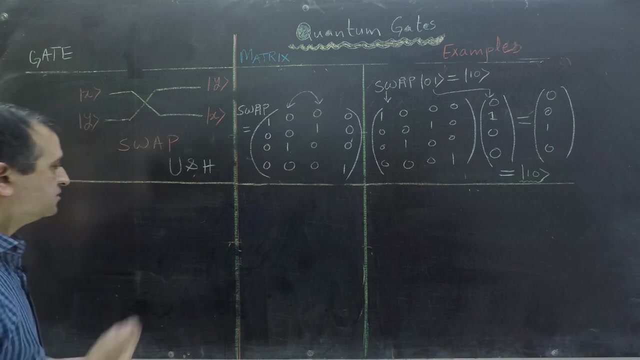 control y gate, control hd gate. So we can take one qubit gate and we can create two qubit control gate using that gate. Let's begin with the c0 gate and then we will see other control gates. So c0 gate, which is also 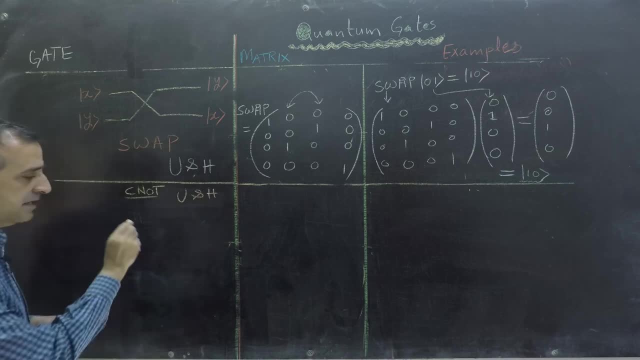 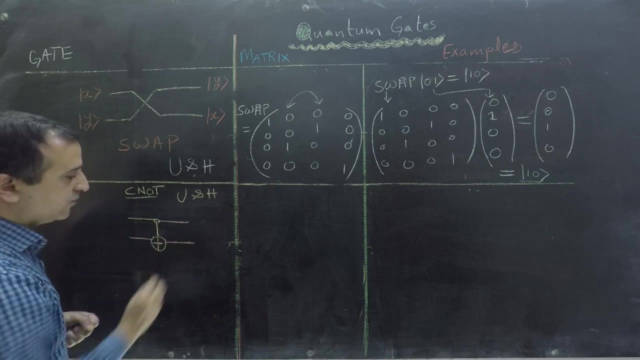 unitary and Hermitian and its diagram is like this: First qubit is controlled and result of first qubit is xor with the second qubit. So if I have x here and ket y here, then my output will be ket x and here I will get. 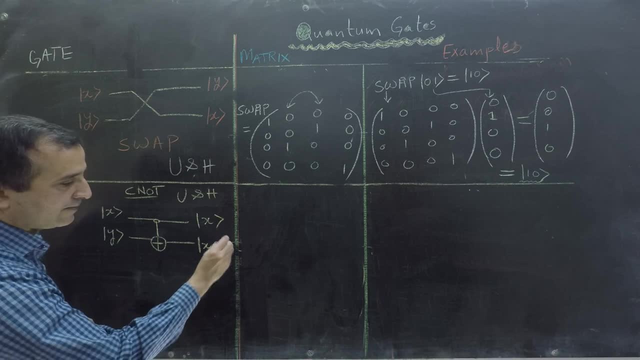 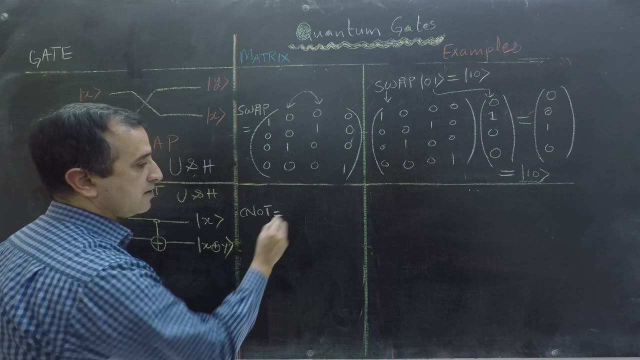 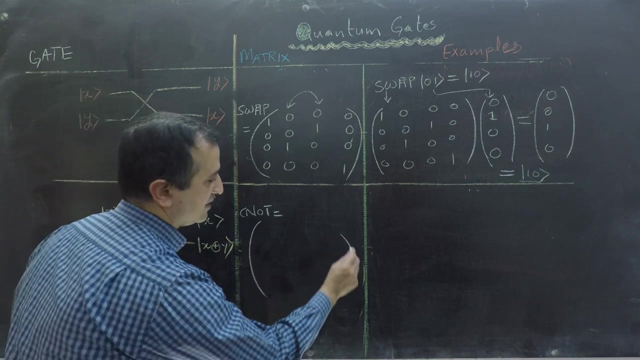 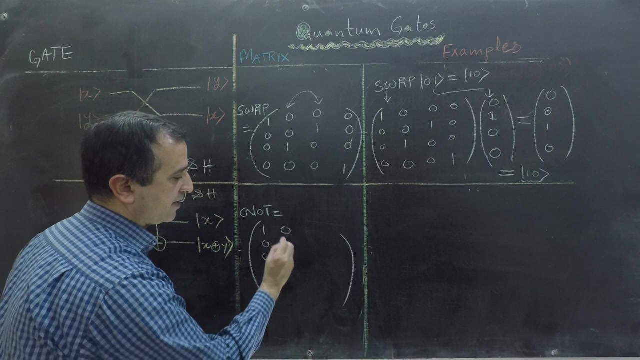 xor with ket y. The matrix of c0 gate is once again a permutation matrix. Permutation matrices are always unitary and Hermitian. In this case my last two columns are swapped, So the first two columns are of identity matrix, but the last two columns 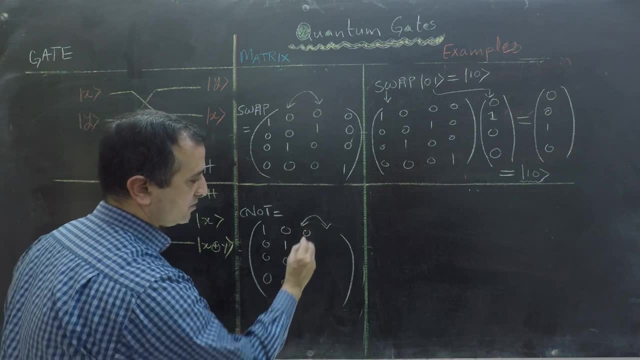 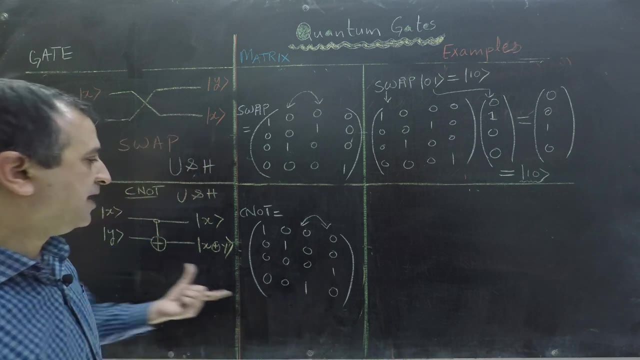 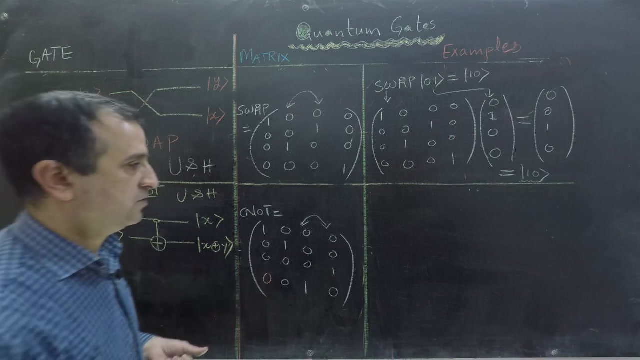 of identity matrix are swapped, So I will get here 0001 and 0010.. That is my c0 matrix and we can try this matrix on any input to find out that this matrix works the way it's supposed to work. So, for example, if I take 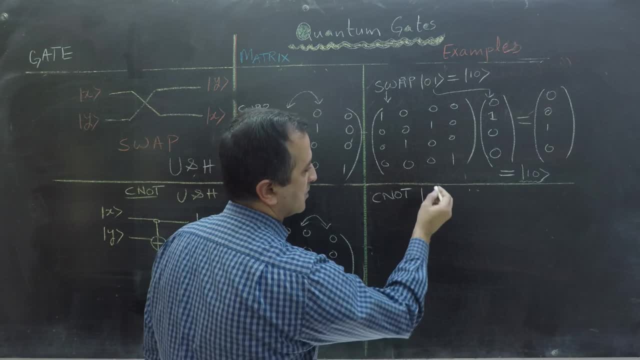 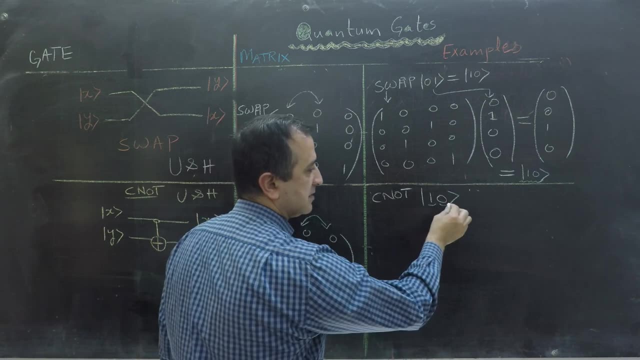 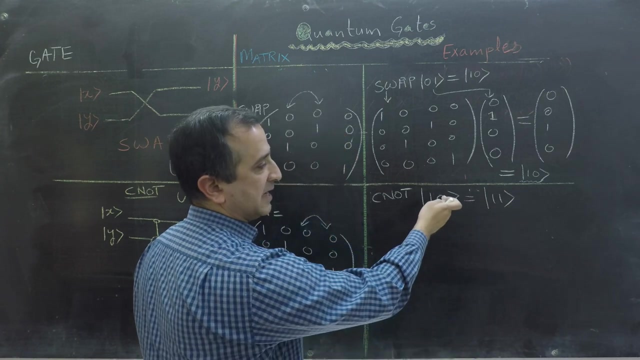 c0 gate and apply it on input 10, because my control bit is 1.. Therefore, this will change, So my answer will be 11.. So whenever my control bit is 1, the second bit is flipped. What about this case when my control bit is 0?? 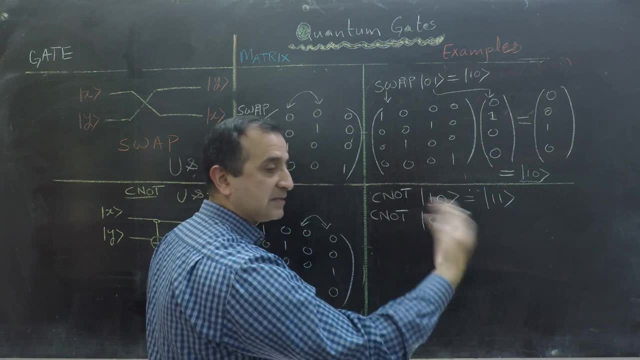 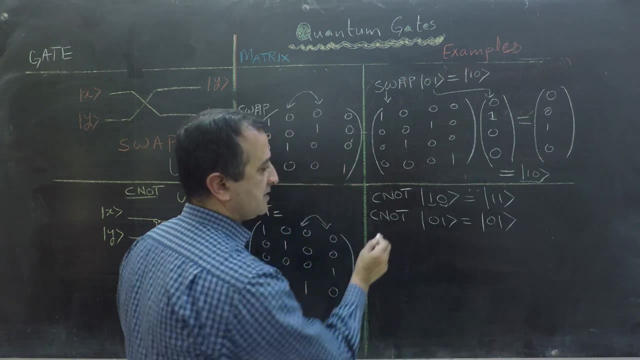 Let's say my control bit is 0, then the second bit remains the same. So my control bit is 0, the second bit remains the same. So, similarly, there are other cases and I have a separate video about c0 gate so you should go and watch. 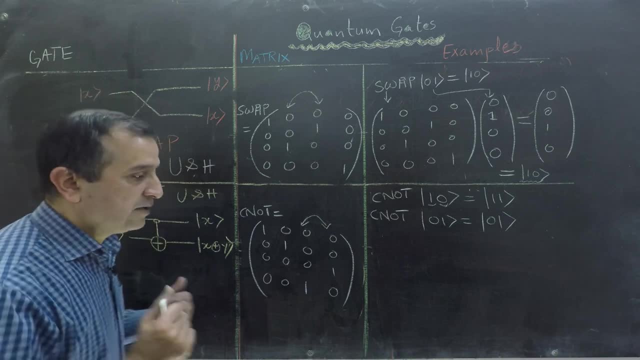 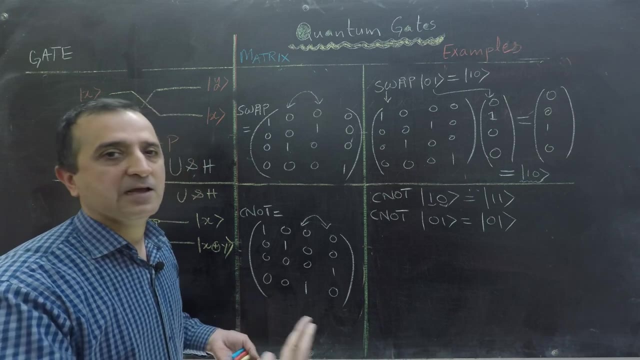 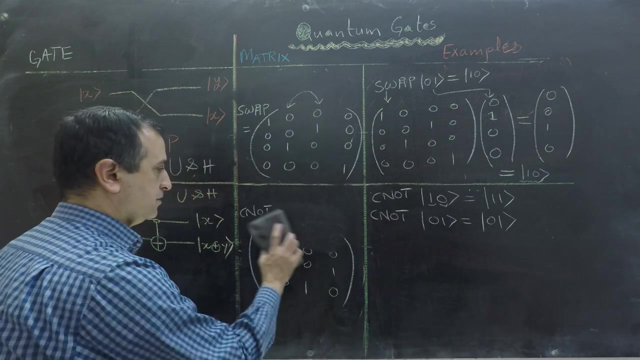 that video also. Now there is an important thing that I want to mention: that we can make control gate out of any single qubit gate. So our formula of making control gate is as follows: But this formula works for big Andean system, For little Andean system. 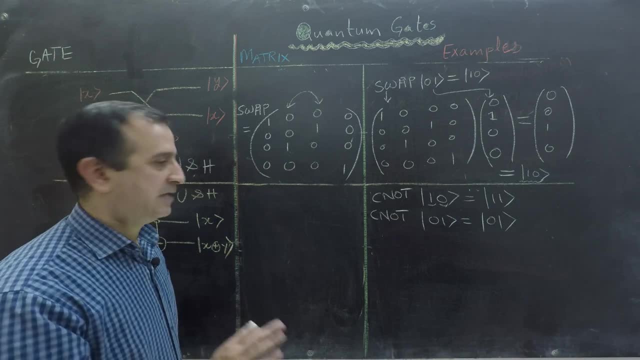 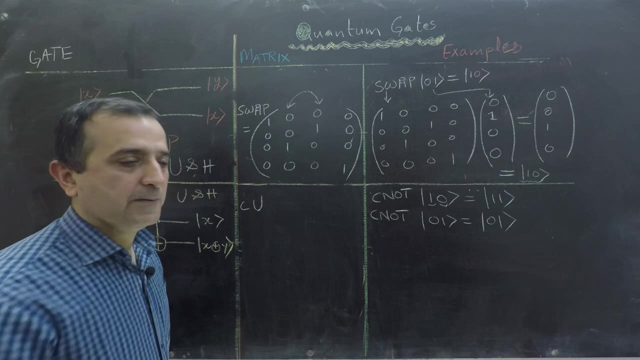 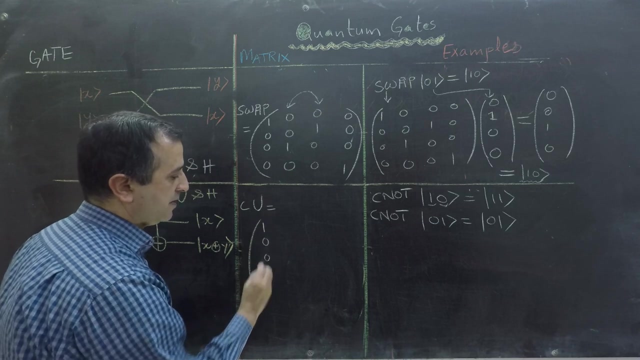 you need to write a different formula, But I like the big Andean system. So let's say I want to make control u gate where u is a single qubit gate. Then my matrix will be that first two rows will be of identity matrix. 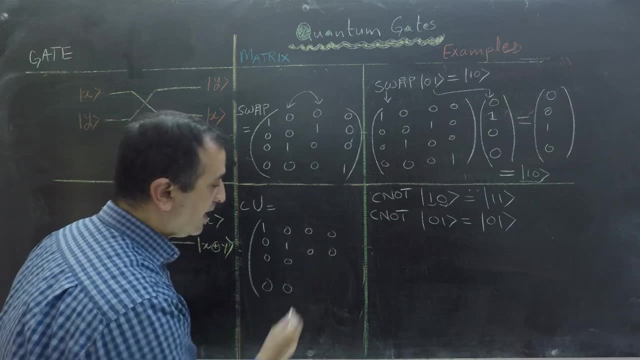 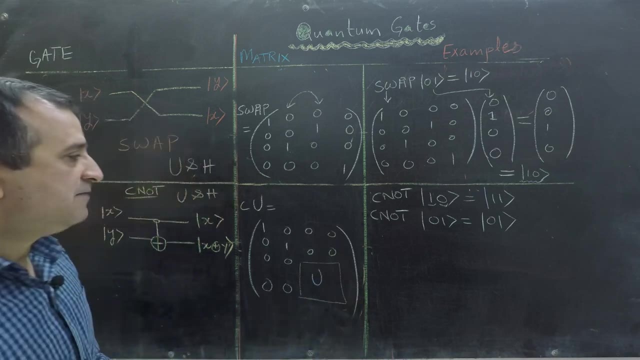 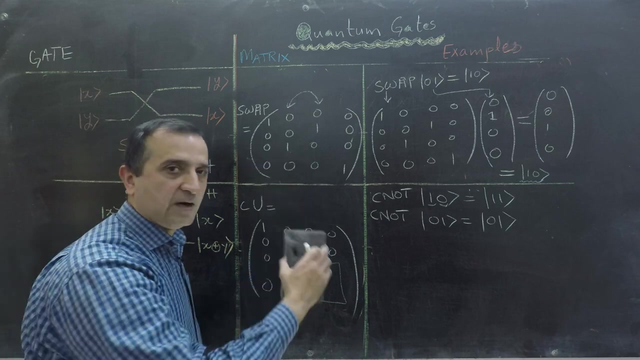 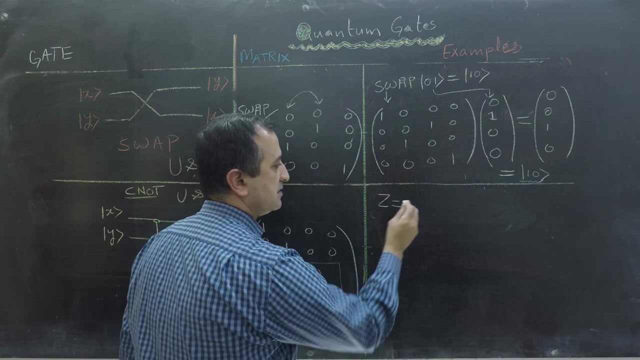 and here I will have four zeros and then here I will have my matrix u. For example, if somebody asked me to make control z gate, I know from the previous blackboard that my single qubit z gate is equal to 1 0 0. 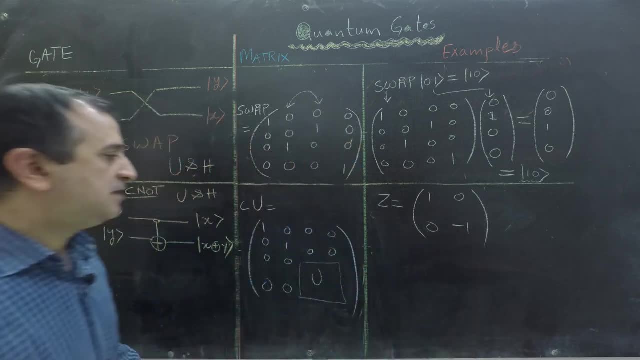 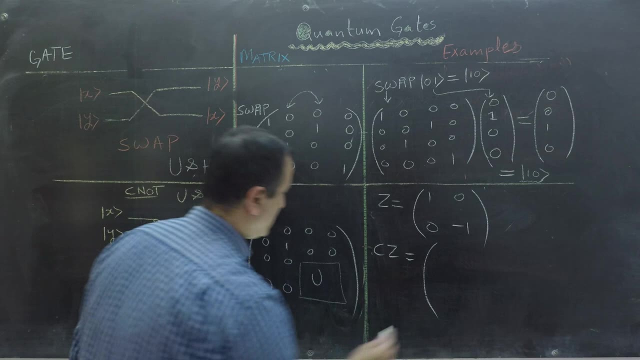 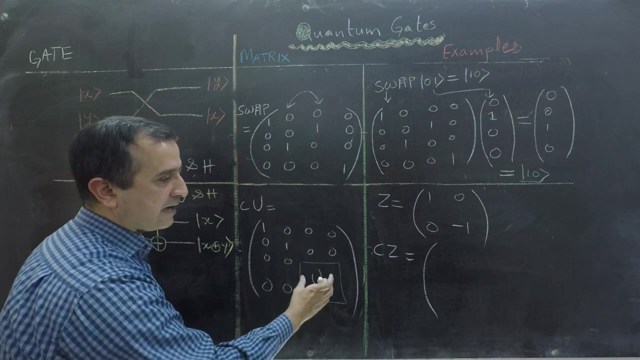 minus 1. So if somebody wants me to make control z gate, then that will be 1 0 0 minus 1, and here I will have 4 zeros and here I will have z matrix. So my result will be 1 0 0 0. 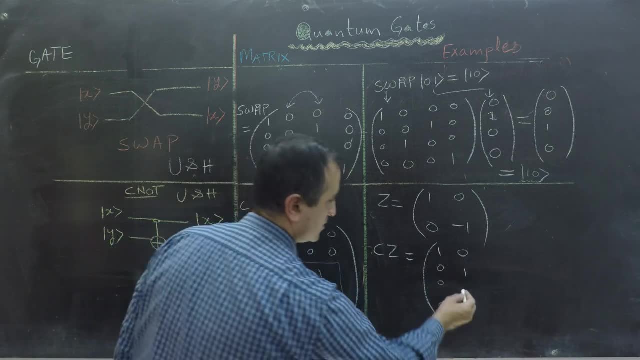 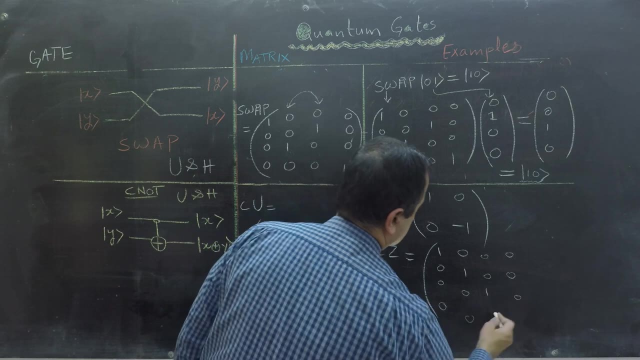 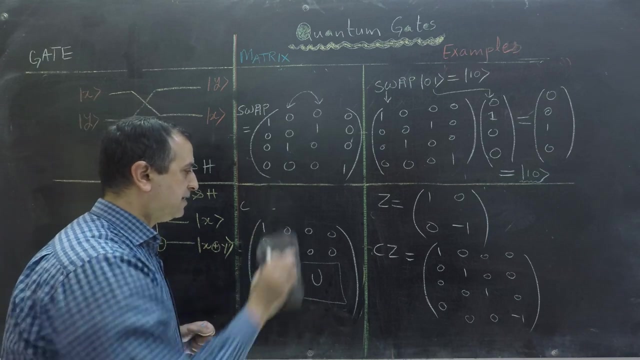 0, 1 0 0 and 0, 0, 0 0. and now here I will have z matrix: 1, 0, 0 minus 1.. If somebody asks me to make control z gate, so how to make that gate? 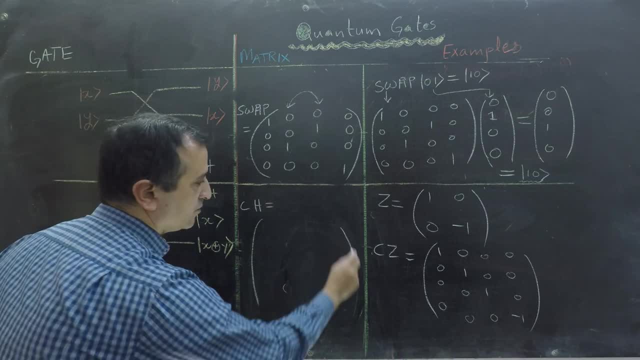 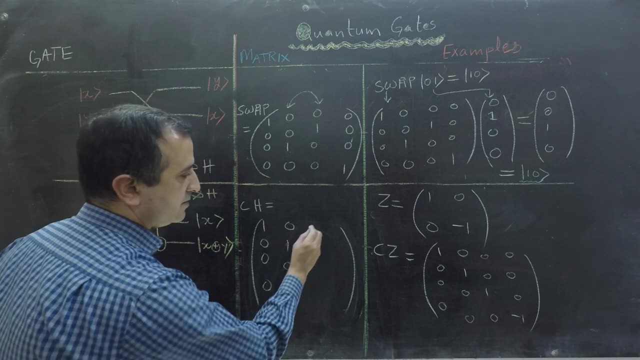 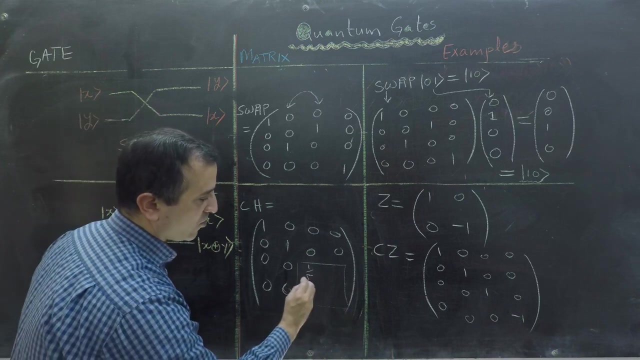 Once again control hadamard gate. I write first two columns of identity matrix: 1 0 0, 0, 0, 1 0 0, and here I will write four zeros. and here I will write my hadamard matrix, which is 1 over square root of 2. 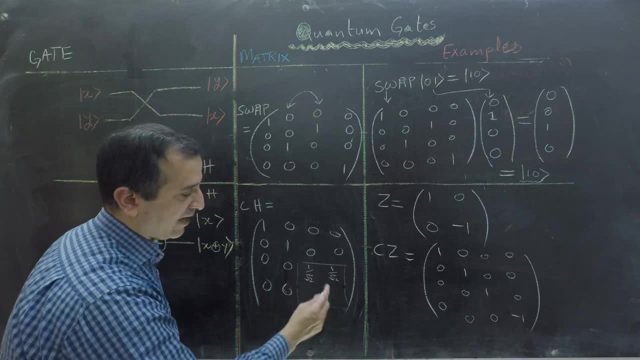 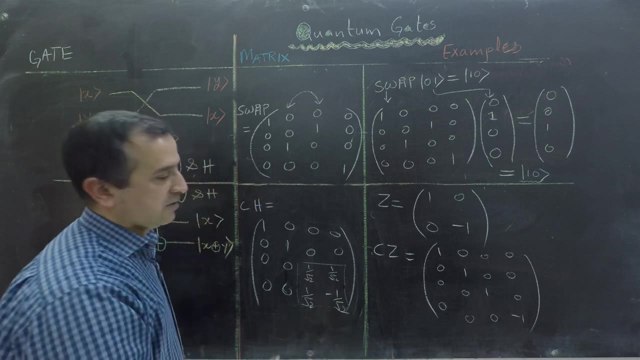 because it is only in these entries. so I have to write 1 over square root of 2, now 1 over square root of 2 and minus 1 over square root of 2. so we have learned a swap 2 qubit gate and we can make many. 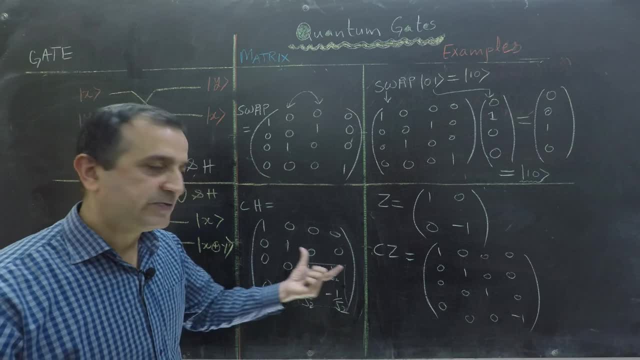 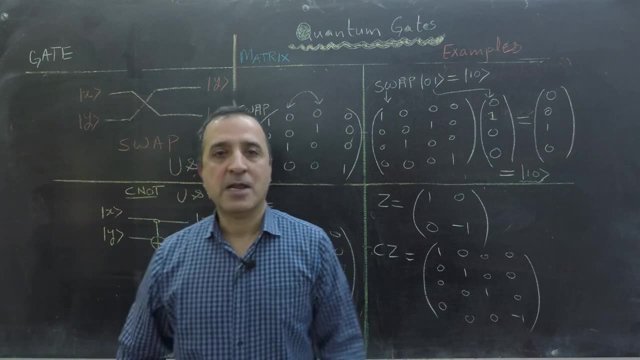 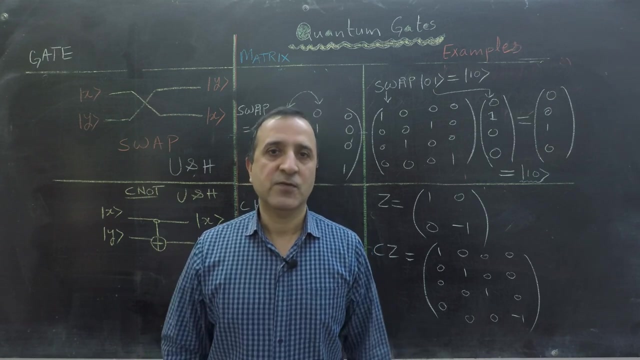 controlled 2 qubits gate using this trick, and one of those gate is c node gate, for which we have separate video, although there are many other quantum gates, but I think for this video these many gates will be sufficient. see you in the next video. bye.